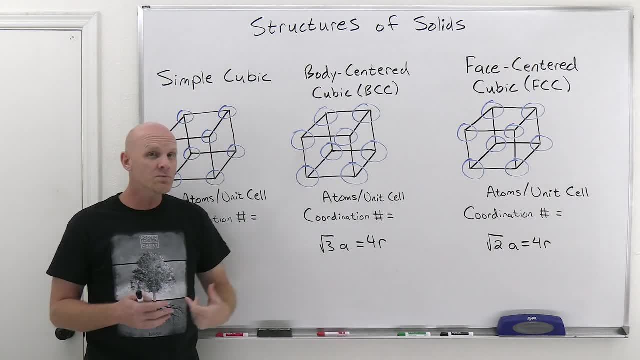 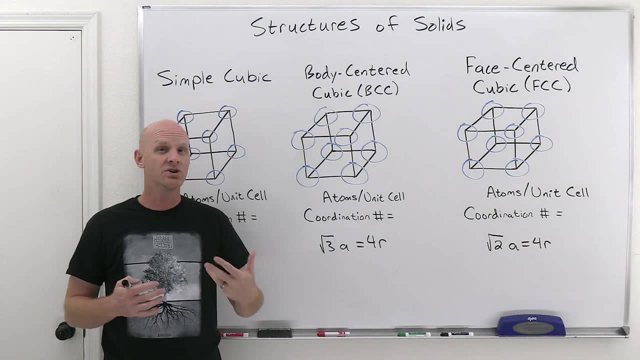 know. what makes it a cubic unit cell is that a cube is the basic repeating unit in the pattern. So it turns out that most solids are going to follow some sort of unit cell in some sort of repeating fashion. Now, not all, though, It turns out. the only mention I'm going to make of it is: 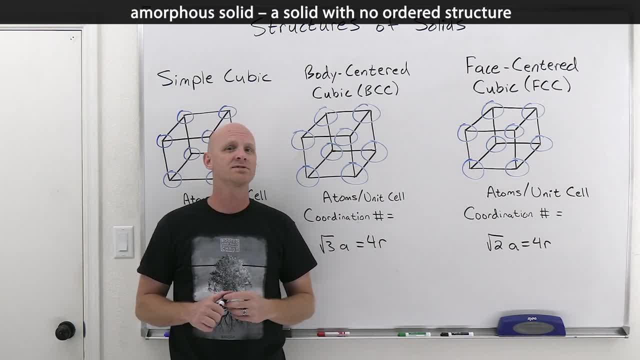 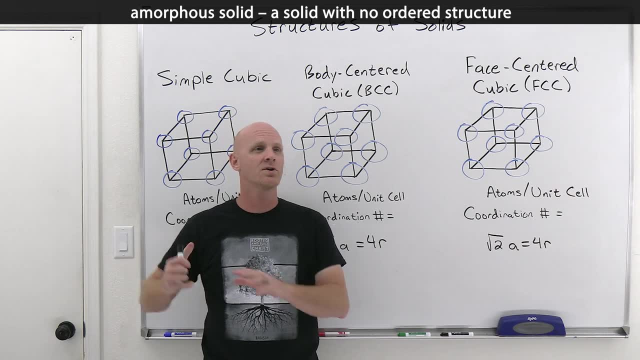 there are amorphous solids, and glass is a good example of an amorphous solid, where there actually is not a regular repeating pattern to the crystal structure. But that's all I'm going to do is mention it. Everything else we'll talk about in this chapter. 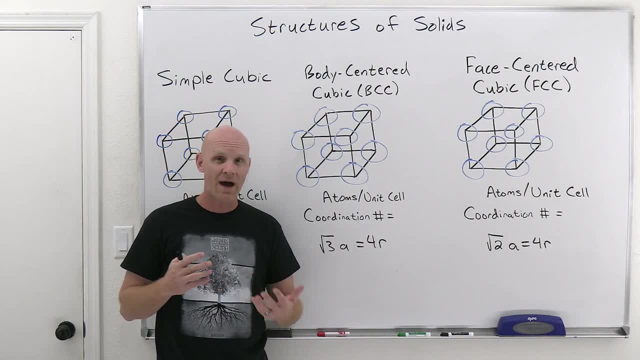 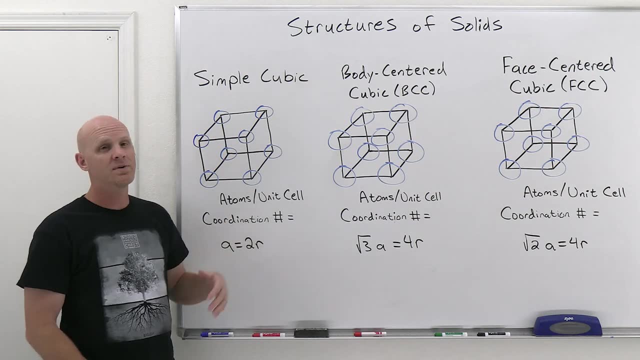 now is going to be some sort of repeating pattern in the crystal lattice structure, And so we'll start with these cubic unit cells And in a cubic unit cell. so again, your basic repeating pattern is going to be a three-dimensional cube And you will always have atoms at the 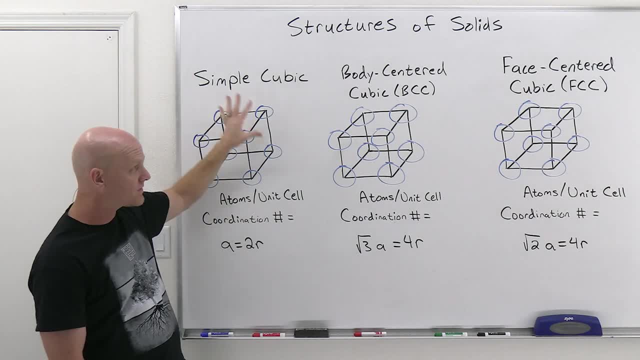 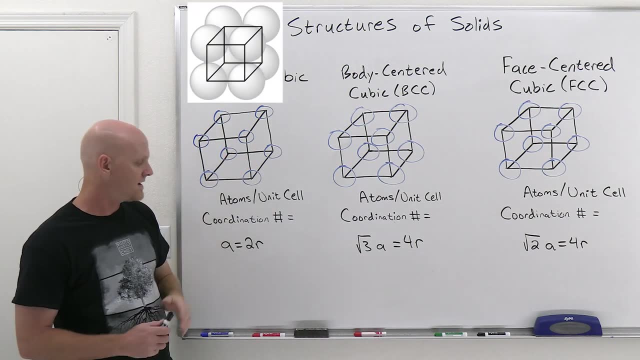 eight corners of that cube, in both the simple cubic, body-centered cubic and face-centered cubic. Now, in the simple cubic, that's the only place you're going to have atoms is in those eight corners. In the body-centered cubic, in addition to the eight corners you're. 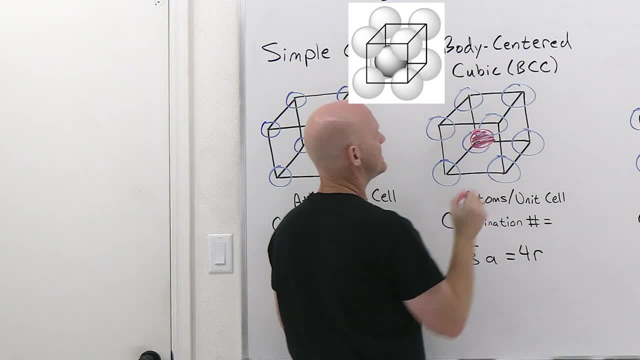 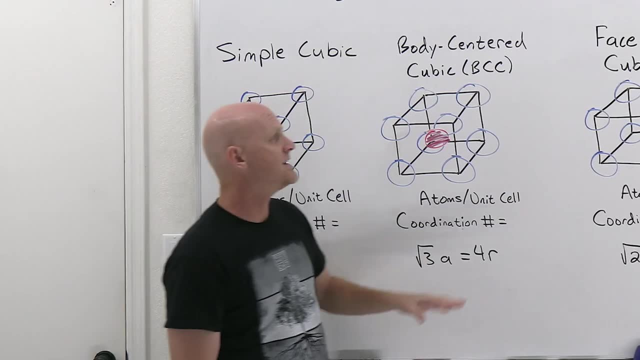 then going to have one right in the very center of the cube, which is hard for me to draw three-dimensionally here, but it's in the very center of the cube, not touching any of the edges and stuff, And then finally in the face-centered cubic, in addition to 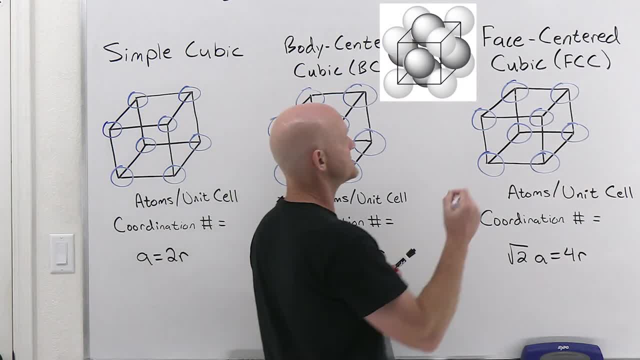 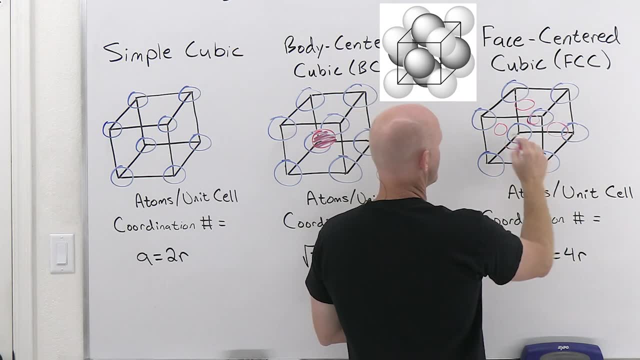 the corners of the cube. again, you're going to have them at the sixth face-center. So you're going to have one here at the top face, one on the left face, one on the right face, one on that back face, one on the front face and then one on the bottom face. 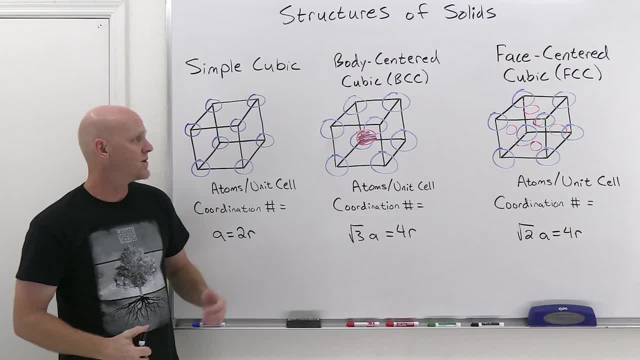 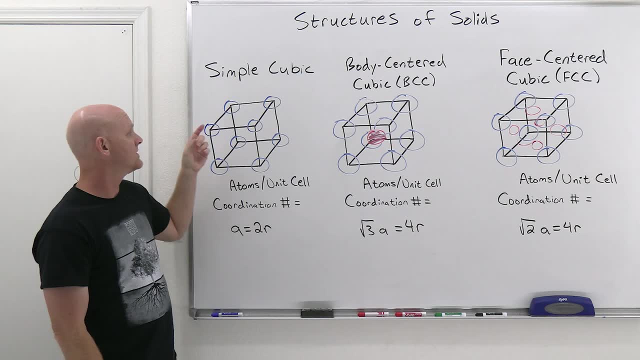 Now, if we take a look at these different atoms here, so in the different positions they contribute a different number of atoms to the unit cell. So if we look at the corners, first off that they all have, so each corner is actually shared by eight different unit. 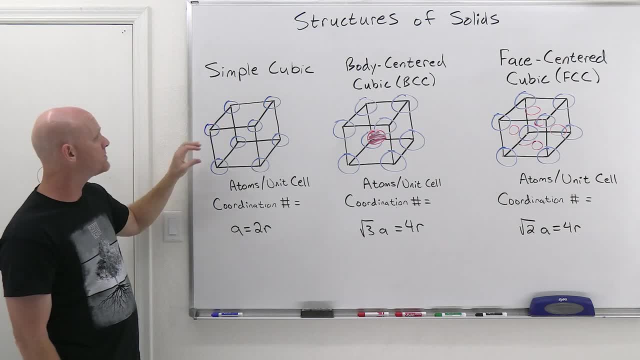 cells. So this corner right here is part of this unit cell, but it's also part of the one to the left of it and the one out in front of it and the one kind of catty-corner out to it right down there. They all share this as kind of one of their upper corners. 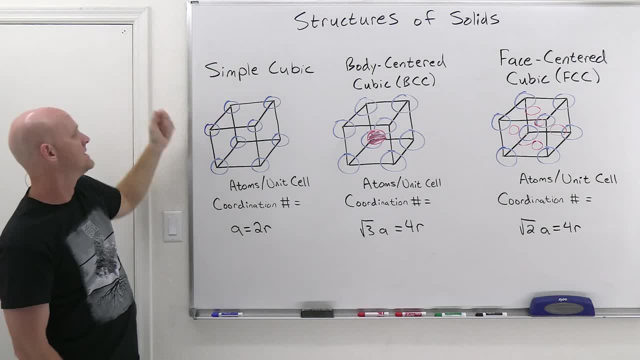 But also you have four more unit cells in the next layer up, so that also share it as one of the bottom corners in their unit cells, And so eight different corners all share, I'm sorry, eight different unit cells all share that corner, And so it. 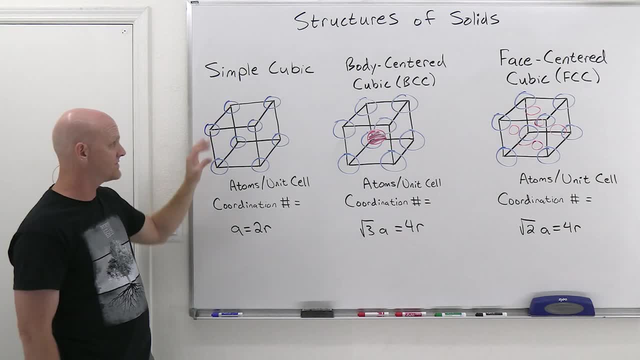 turns out, only one-eighth of that atom is in any one of those unit cells, And so in the unit cell we've drawn, only one-eighth of the atom's volume is actually in this unit cell, And so we say that each of the corners contributes one-eighth of an. 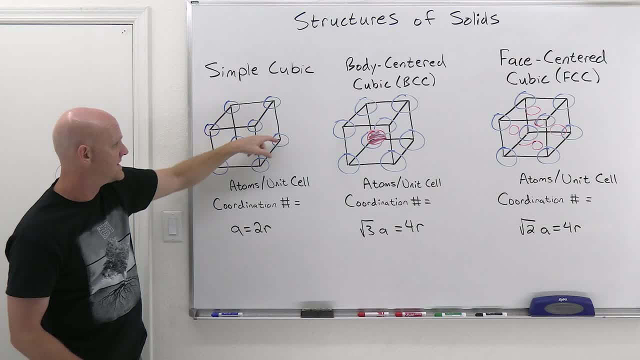 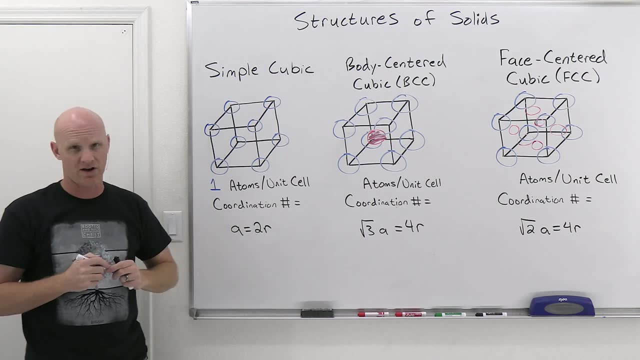 atom. And so for the simple cubic with just these eight corners, each contributing one-eighth of an atom to the unit cell, we say there is just one atom per unit cell, So, and it's not one atom in any one place, but there's an eighth of an atom. 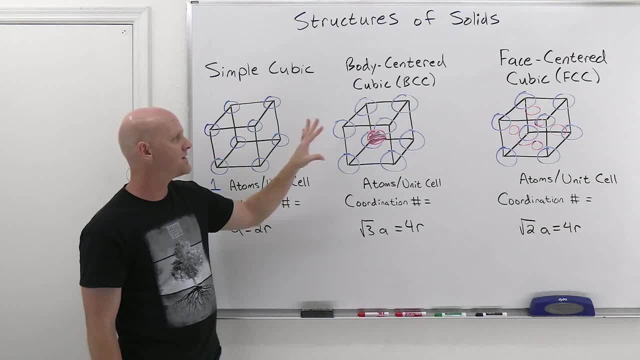 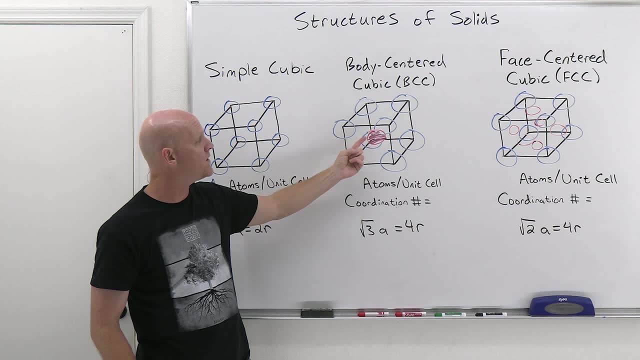 at eight different corners. Now if we move on to talking about the body-centered cubic unit cell again, we still have those eight corners and that's eight times one-eighth. again is one atom per unit cell, but we also have one at the body. 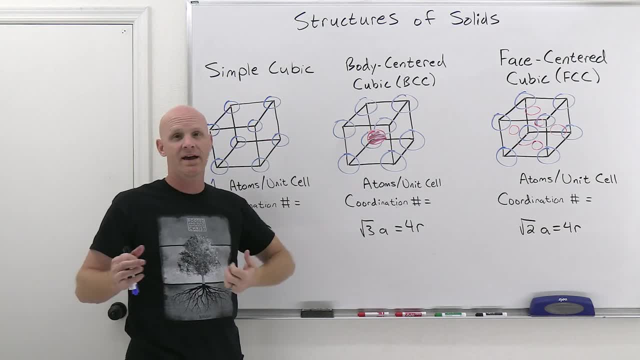 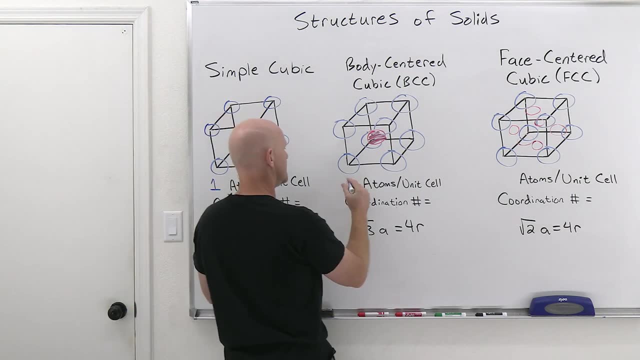 center, in the very center of the cube, And it's not shared by any other unit cells, so like the corners are, And so in this case that contributes one additional atom, and so we have a total of two atoms per unit cell. Again the eight corners contributing one-eighth each. that's 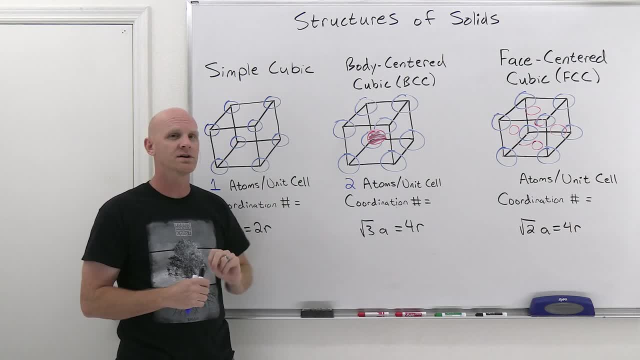 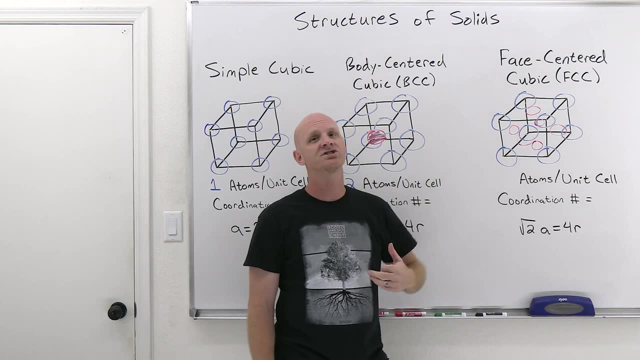 one atom per unit cell plus the body-centered position gets us to a total of two atoms per unit cell. And then finally in the face-centered cubic. so the ones that are in the face centers are shared between two unit cells like this: 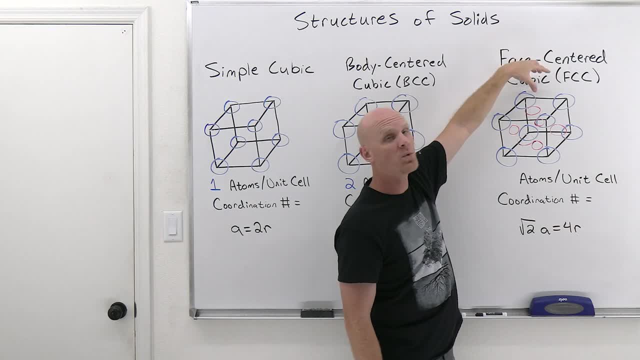 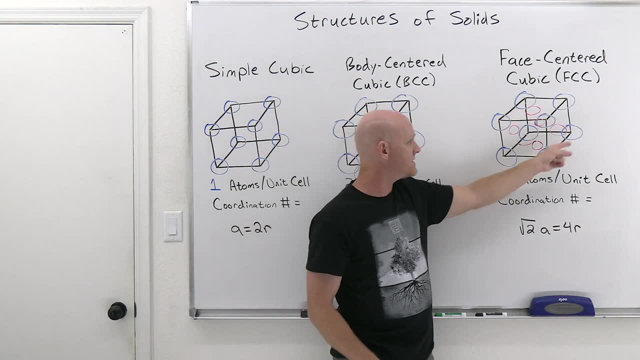 one on the top face is shared between this unit cell and it's shared by the one right above it, and so that atom right there is half in both of those unit cells, And so in this case with six different face centers each half. 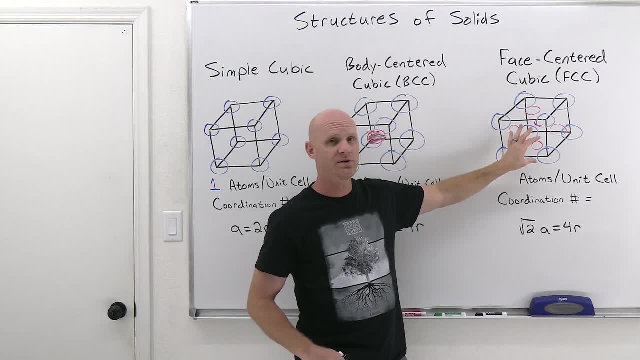 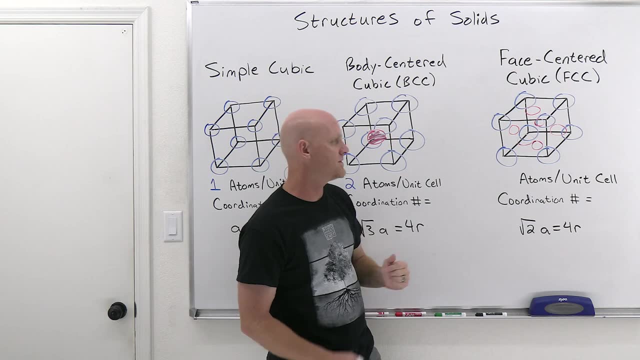 times a half is three. That's going to contribute three atoms to this unit cell for the face-centered positions, and then the corners, yet again, are going to contribute one more atom per unit cell, like it did in the other cubic unit cells for a grand. 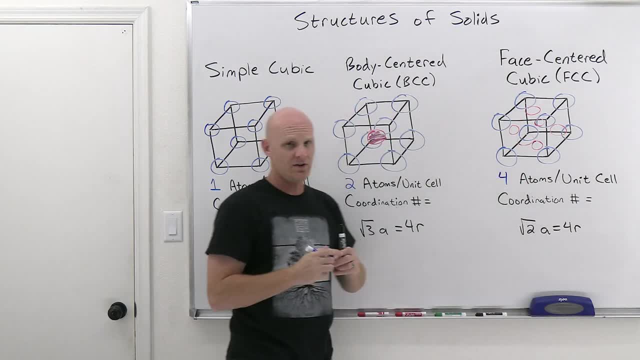 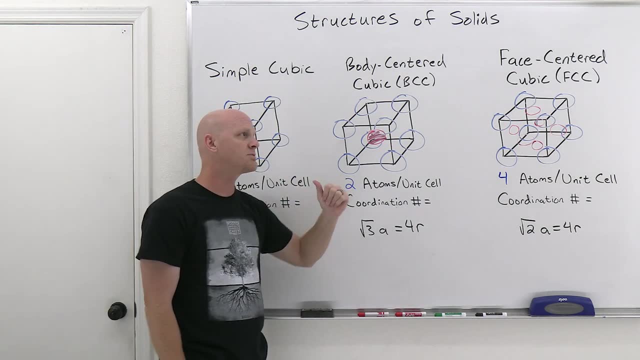 total of four atoms per unit cell. And so this is, you know, one of the characteristics you're supposed to memorize for these unit cells: Simple cubic: one atom per unit cell. Body-centered cubic: two atoms per unit cell. Face-centered. 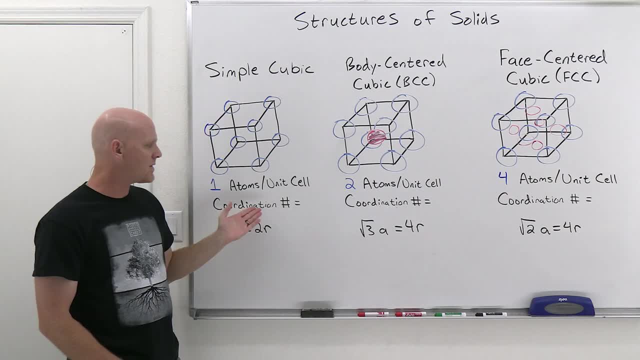 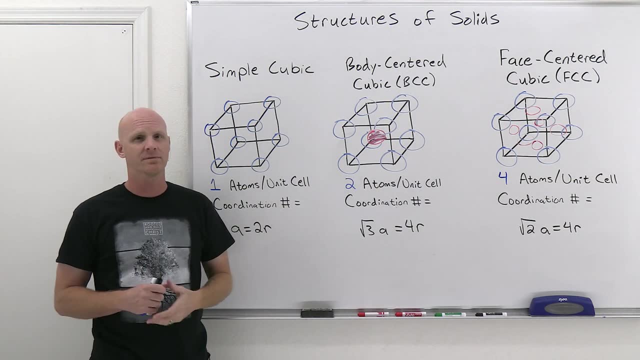 cubic: four atoms per unit cell. Now we also talk about what's known as the coordination number, and the coordination number is just the number of nearest atom neighbors to any given atom in the structure. So if we take a look in the simple cubic, so if I look at this, 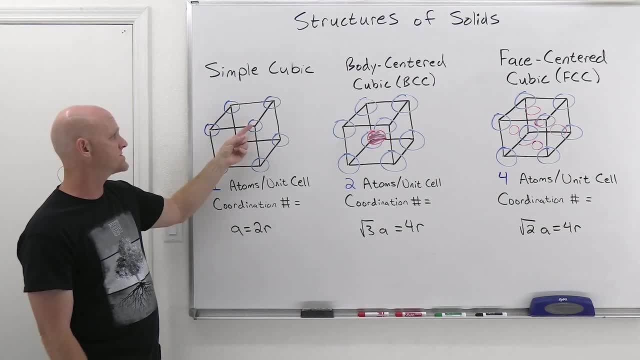 corner. here the nearest neighbors are the adjacent corners, So there's one behind it and there'd be one in the next unit cell out in front of it. There's one to the left and there'd be one to the right in the next unit cell. 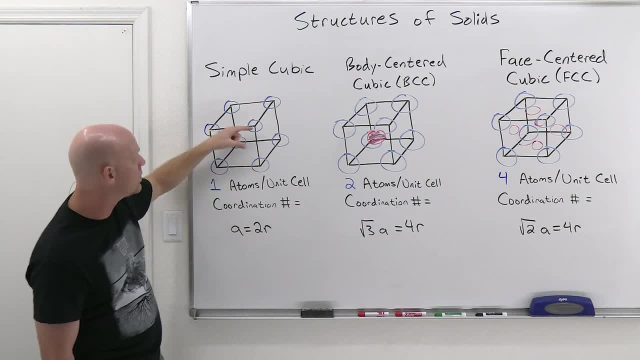 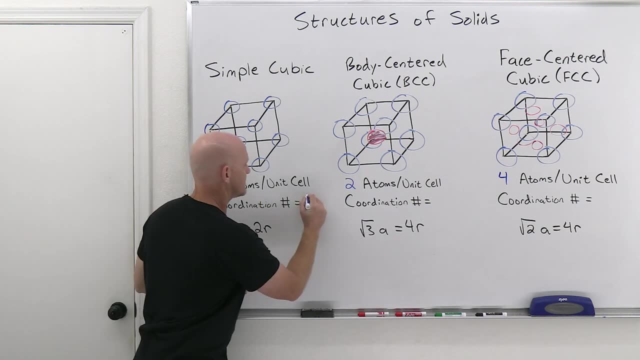 not drawn in, And then there's one below it, and then there'd be one above it in the next unit cell there, And so it's in all six directions. there's going to be a nearest neighbor, and so we'd say that the coordination number here is going to. 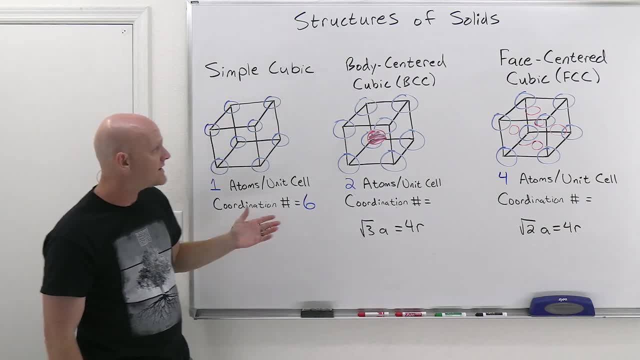 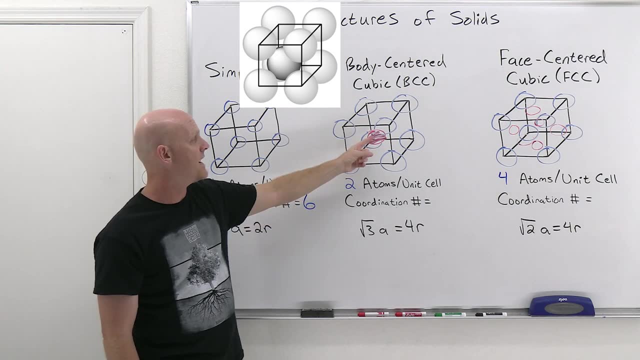 equal six in the simple cubic unit cell. Now in the body-centered, this one's going to be a little more difficult to see for one of the corners, but you can totally see it for the body-centered position. That body-centered position is actually equidistant from all four on top and all four. 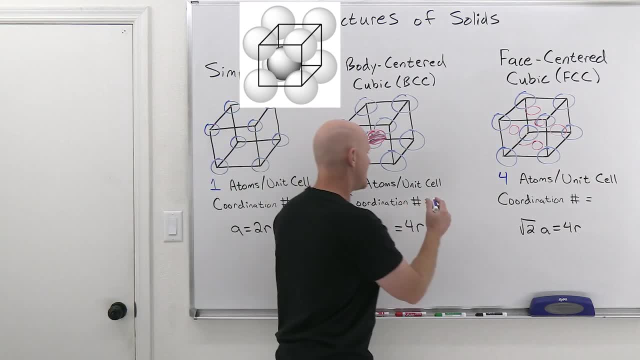 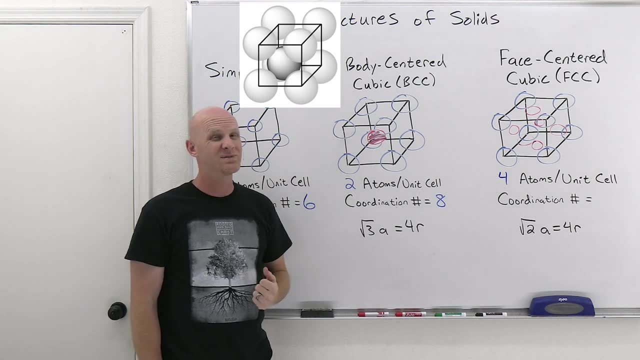 atoms at the corners on the bottom, and so he has eight nearest neighbors and it's going to have a coordination number of eight. Now, if you tried to find what the coordination number is for the corners, you'd still find it to be eight, but it'd be really difficult to see, especially with only 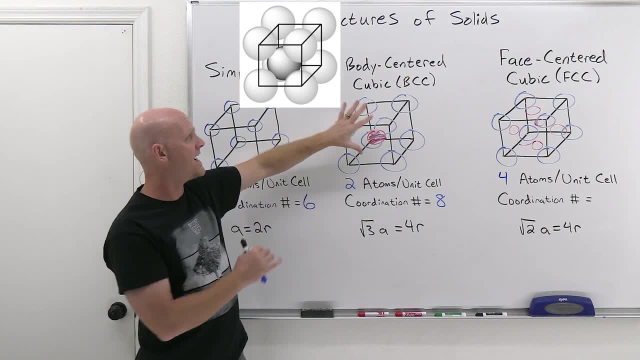 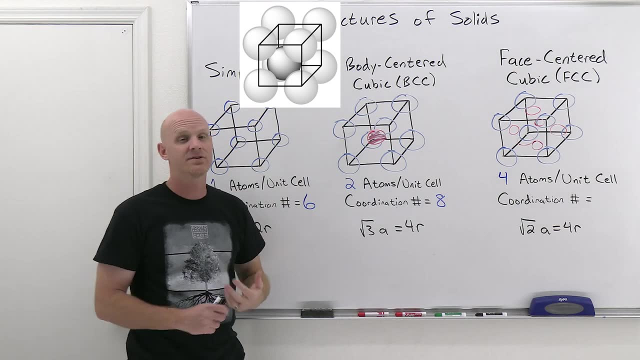 one single unit cell drawn in. But it turns out if you offset the entire body-centered cubic structure you could actually draw another unit cell where this guy was the center of an offset kind of body-centered unit cell and things of this sort, and would still have a coordination. 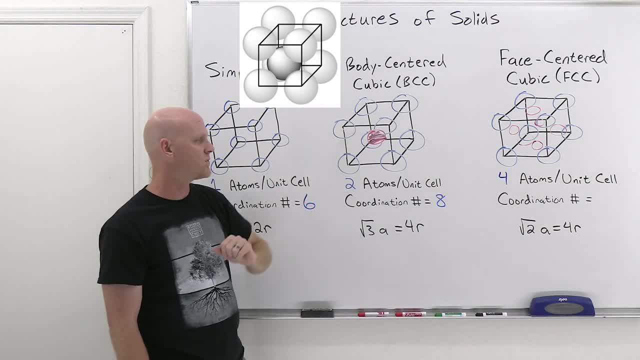 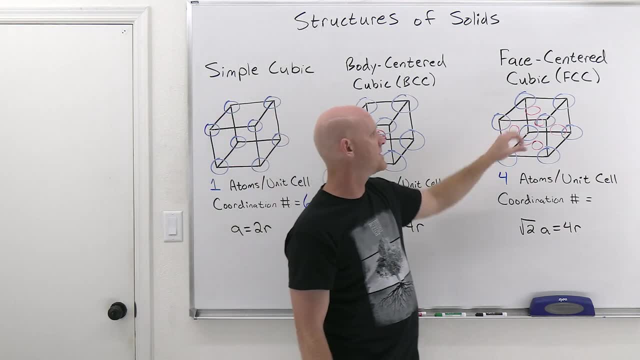 number of eight. Hard to see here, but definitely not too bad to see for the body-centered position, So, but the coordination number for all the atoms is indeed eight. And finally, for the face-centered cubic, this one's going to be a little harder to see, So, but in this case, if we try to, 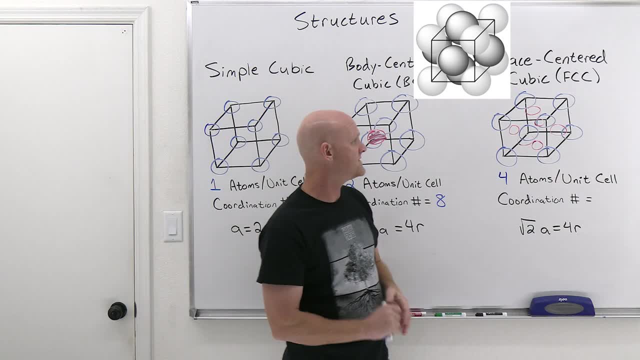 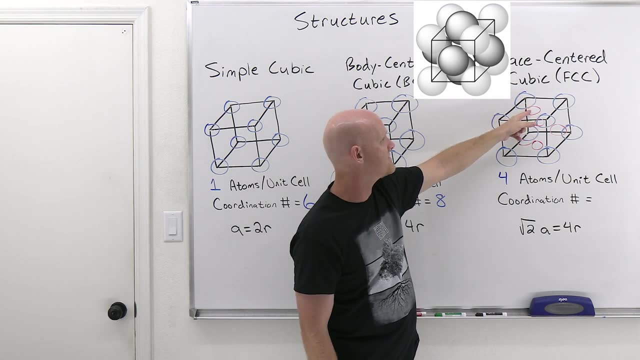 find all of the nearest neighbors. maybe we pick this face-centered position right on the top edge here and so he's definitely got four nearest neighbors on the four on the corners, but it turns out he's also equidistant to the four face-centered positions on the level right. 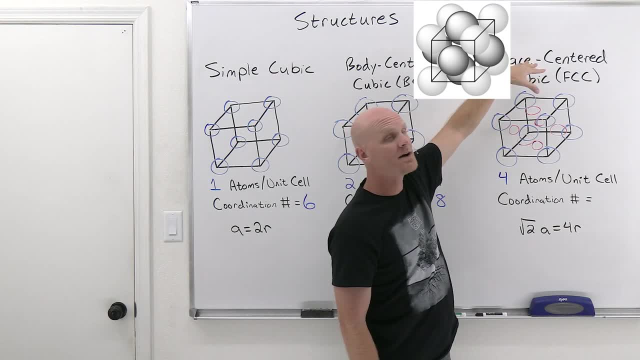 below him and on the unit cell, the four face-centered positions on the level right above him as well. And so it turns out he's got 12 nearest neighbors and a coordination number of 12. And so in that face-centered cubic, 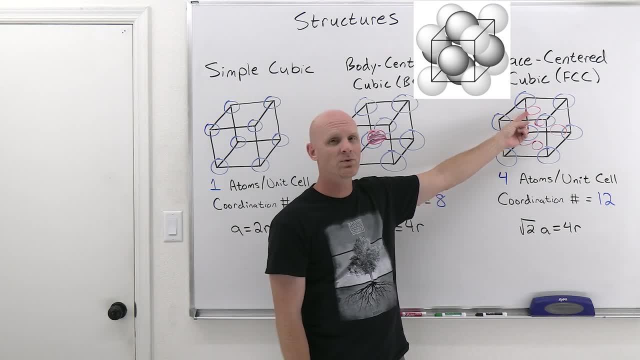 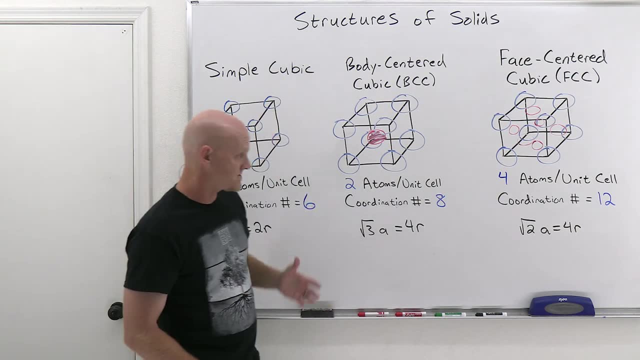 lattice every single one of the atoms. and again it was easiest to kind of demonstrate, maybe for one of the face-centered positions, but it's also true for the positions at the corners as well. Okay, so now we know the number of atoms per unit cell and the coordination. 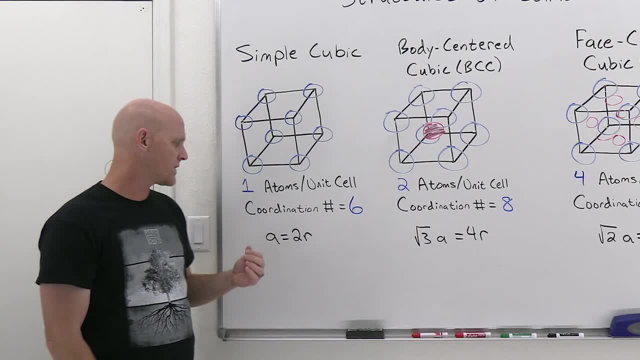 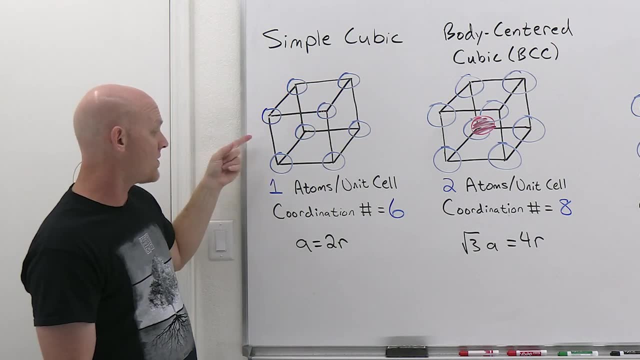 number for each. So, and now we got a little more to talk about and we're going to define the edge length A. So notice that for a cube, all the edges have the same length for a perfect cube here, and they're all going to be called an edge length of A, And it turns out that 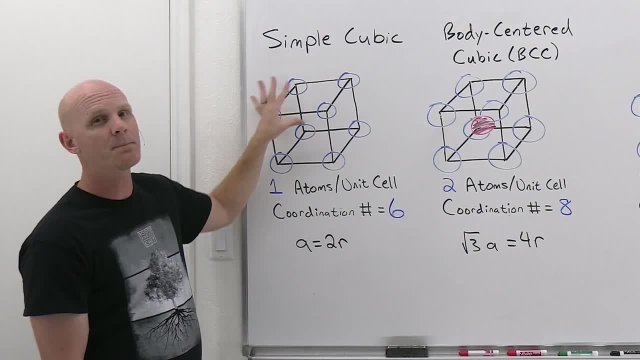 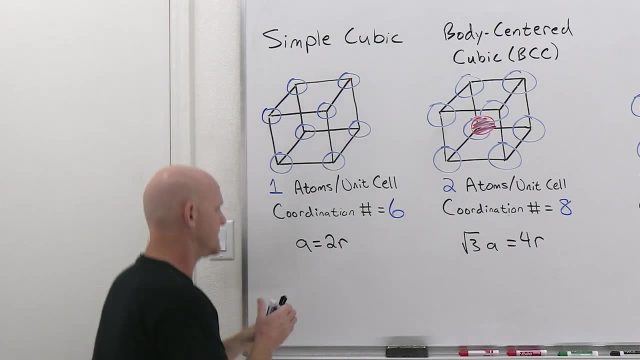 that edge length is going to equal two times the radius. This isn't really drawn perfectly, and it would actually get a little hard to see where all the atoms are if I really tried to make this perfect. but it turns out if we just take one of the edges right here, we'll draw that in a little better, And so just one of 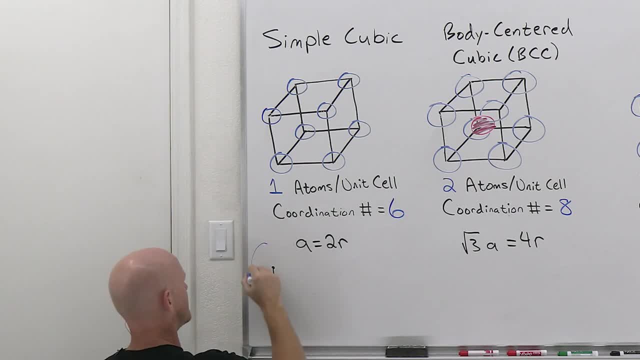 those edges of the cube, it turns out, if you actually try to represent this better, so you actually have the atoms touching as we go across. And so this entire edge length A, it turns out. if you look at it from another perspective, you can see that it's equal to. 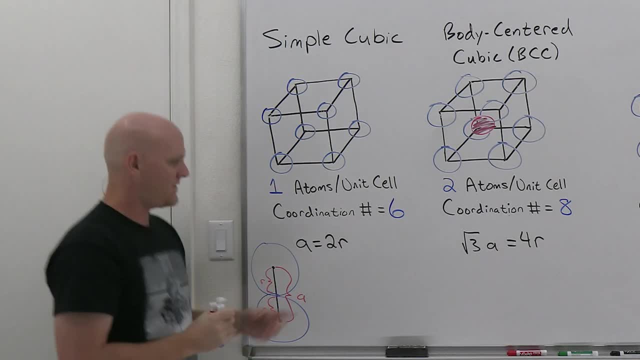 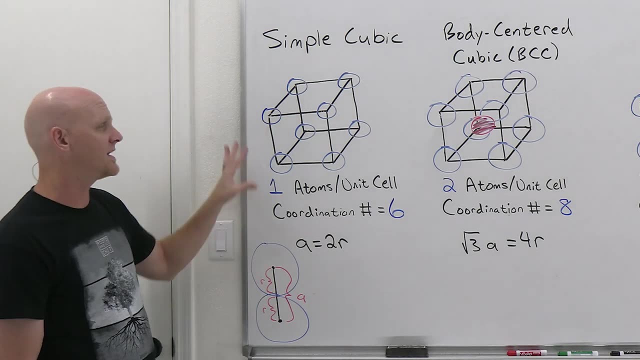 two, Two times the radius of the atoms, And that's where this kind of comes from. That's the simplest relationship. So it turns out right along an edge length the atoms actually are touching. And again, most drawings we'll give you won't actually show them touching. but 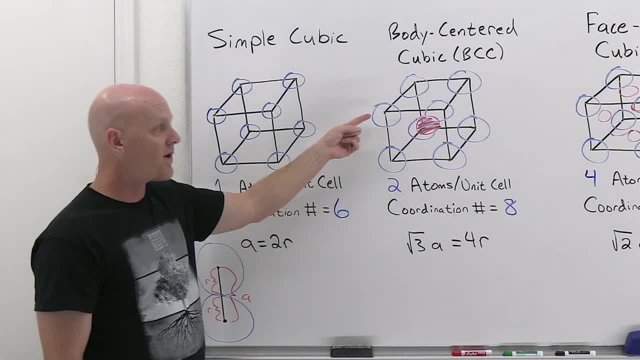 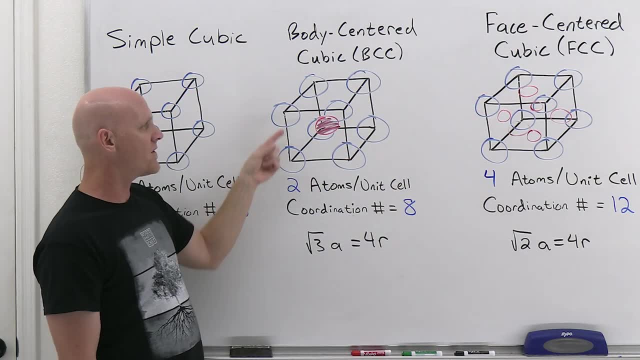 they are Now. where this is going to get confusing is that they actually aren't touching in the body-centered cubic or the face-centered cubic, as I've drawn here, even though they were in the simple cubic, So these atoms aren't actually touching here. In fact, where they're. 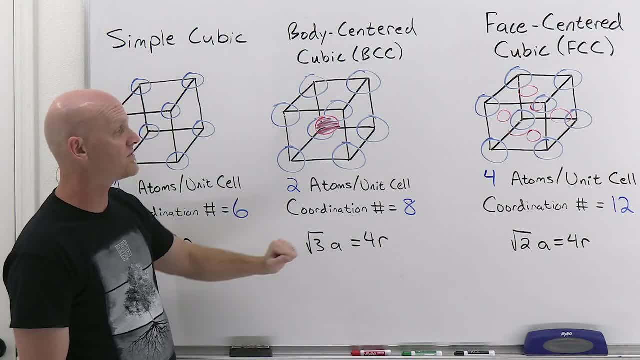 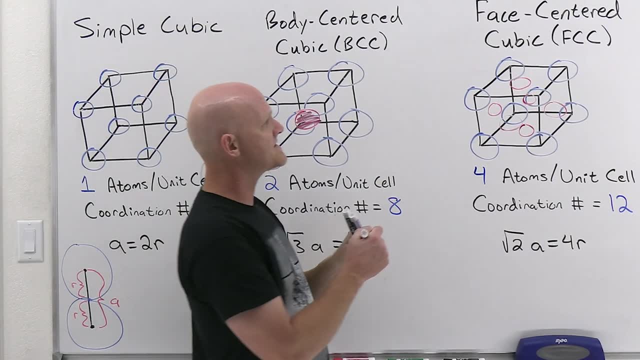 touching is a little more challenging to see And it's actually easier to see. It's easier to see on the face-centered cubic And so we're going to derive this relationship for the face-centered cubic first And so it turns out on the face-centered cubic if 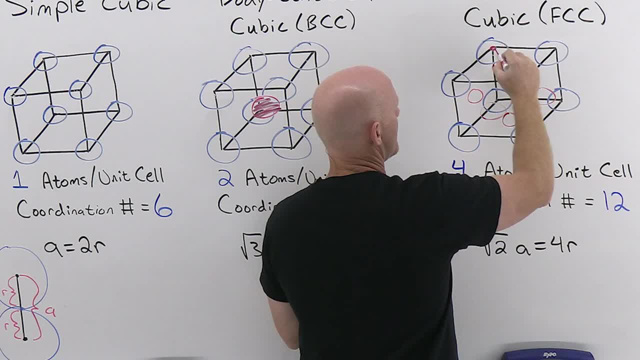 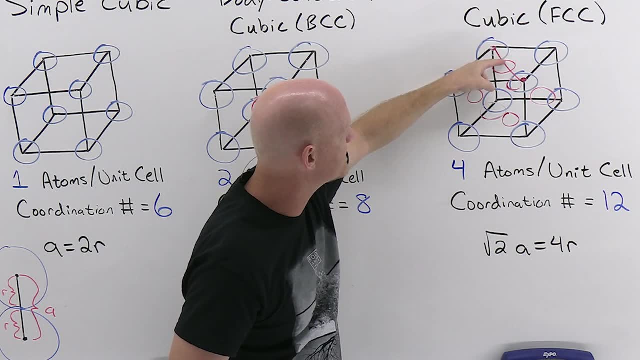 you want to see where the atoms are actually touching. they're touching right across a diagonal on any face And so as you go from one radius here to a full diameter of the face-centered atom, to one more radius here, so right across that diagonal is going to. 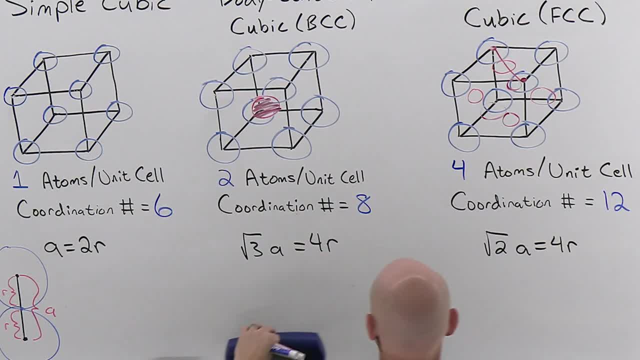 equal four radii. So if we actually try to draw this out just a little bit- So in this case I'm going to draw out that That entire top face- We'll draw that middle atom again And then we'll draw the atoms. 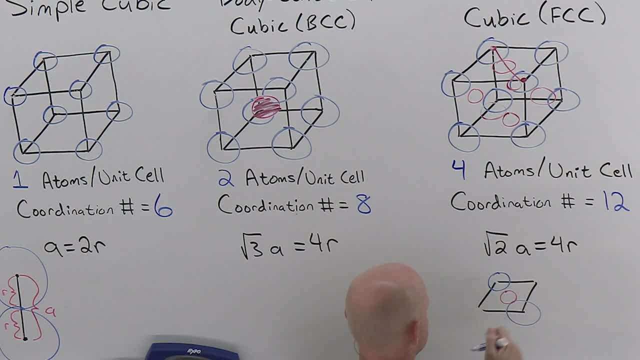 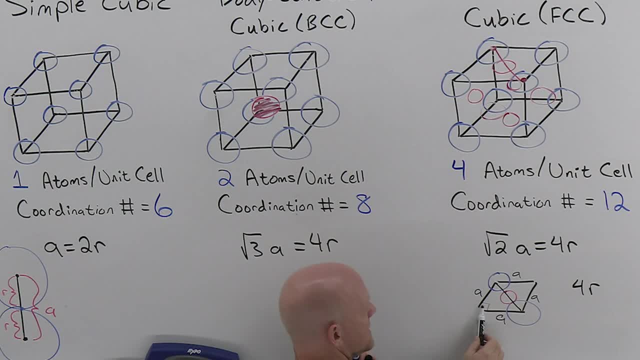 that this is going to be the hypotenuse of a right triangle. So all the angles here are 90 degrees everywhere. So it's the hypotenuse of a right triangle And in this case, with the two sides being A, you get A squared plus A squared equals the hypotenuse squared, And you actually get 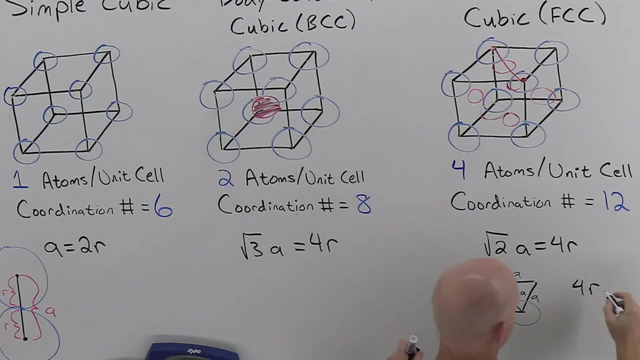 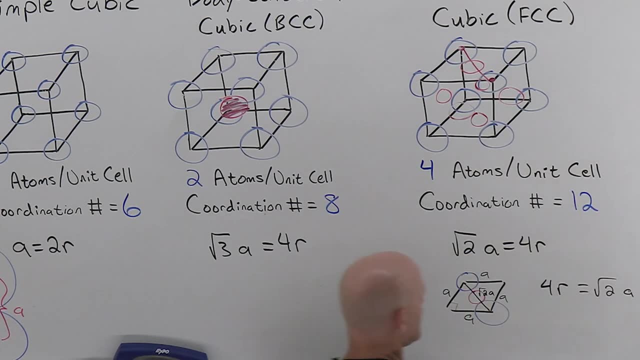 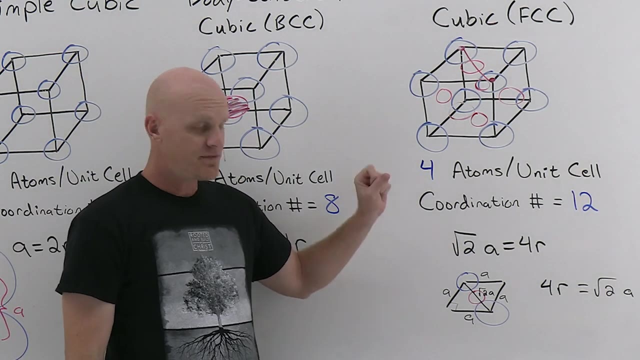 that it's going to equal square root of two times A, And that's where this kind of idea that square root of two A equals four R comes from. So just looking at that right triangle, Cool, Let's go, Okay. So. So if we were to actually use this to calculate packing efficiency, 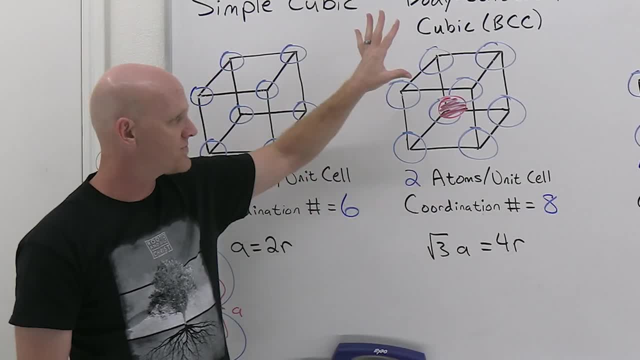 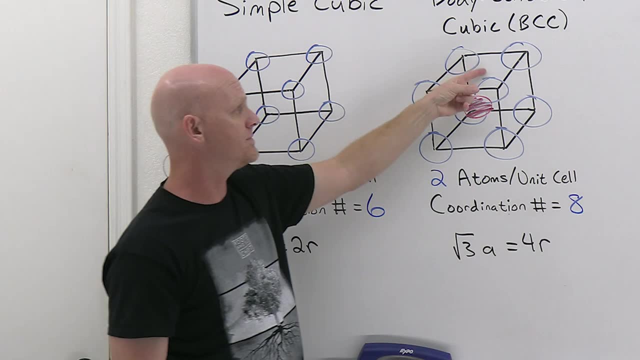 we'll deal with that in just a second. Now, the hardest one to see is for the body centered cubic, because it turns out the atoms aren't touching again along an edge and there's no face centered atom to talk about And these atoms are definitely not touching. So where are the atoms actually all touching? 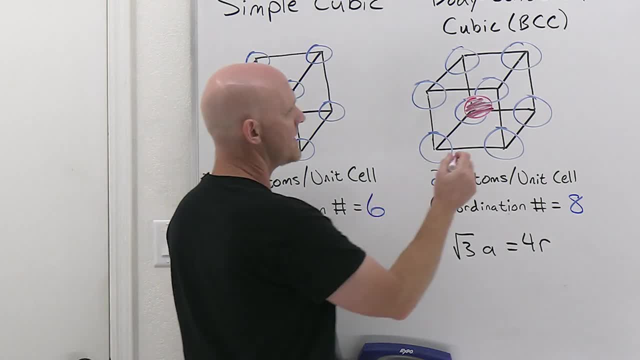 Well, it turns out they're touching along a body diagonal. So if you went from one of the lower front corners to the exact opposite corner in the back, We're going to find out who our upper-lowerster geometry average is. And then, of course, what we don't know is: 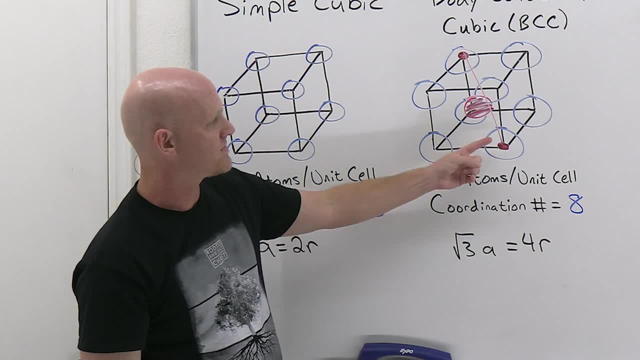 what our left-left�level democrats are, and then workers in the right lovers. They're going to find that value for body. So we're going to built a hard Teilic, We're just going to. atoms would be touching, And so this atom in the corner would actually touch the one in the body. 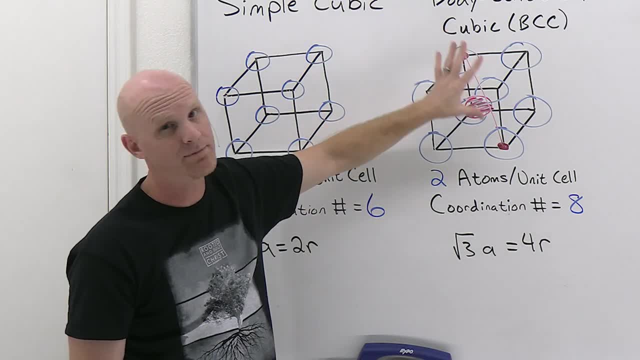 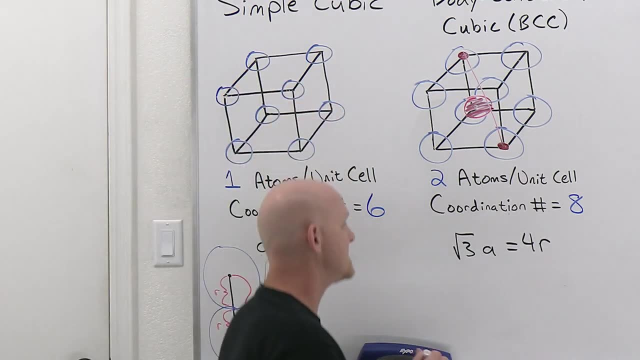 center and that body-centered one would be touching the one in this corner which, again, my drawing doesn't show, But again, if I actually tried to show it it would get a little bit confusing. The one that's in the study guide is a little better in that regard. So if we take a 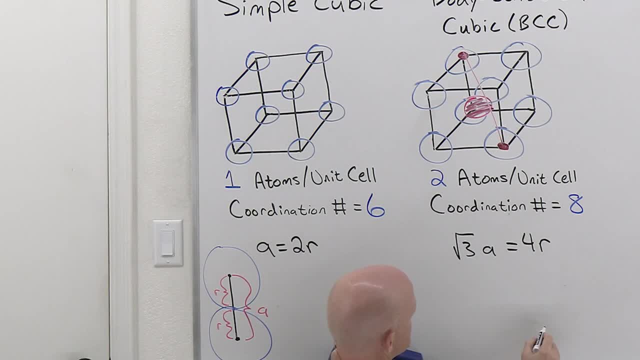 look at what's going on here and we're just going to kind of, in this case, draw a right triangle where this is our 90 degree angle And in this case, so this is going to correspond to this right triangle right along here, up the backside and then right down the top. 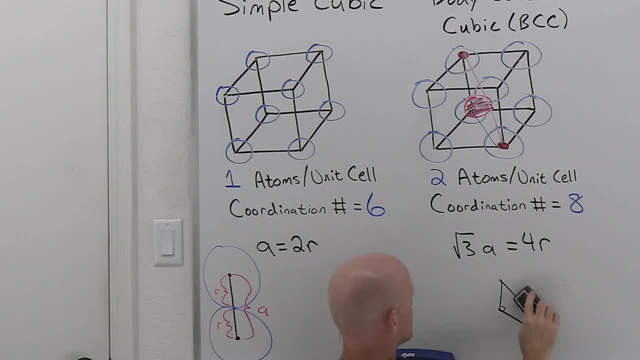 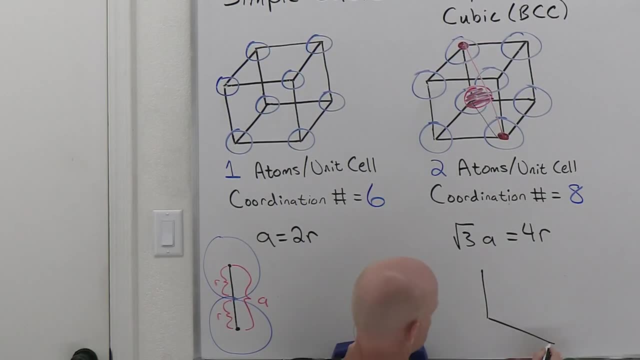 And so maybe actually we do this in red to make that make a little more sense. In fact, let's try this one more time And again. this would be a right angle here. So this is edge length, A right up the back. 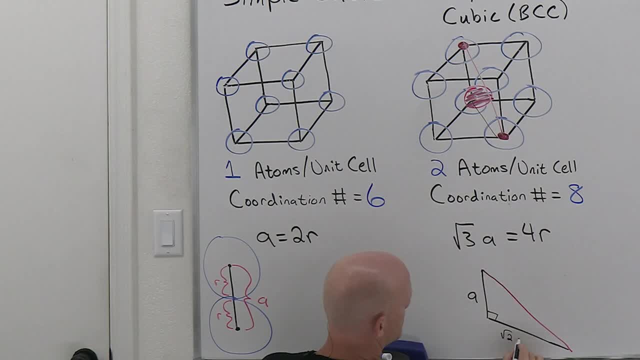 This is going to be one of the face diagonals which we already figured out was equal to the square root of 2A And then if you get your A squared plus B squared equals C squared here. so you'd have your A squared plus the square root of 2A. all squared is going to be 2A squared. 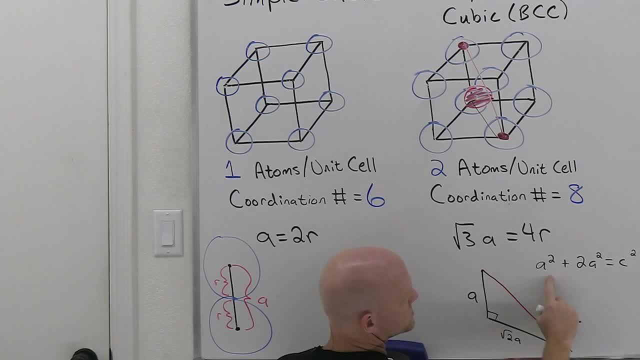 equals your hypotenuse squared, And so it'd be 3A squared equals C squared. So C here is going to equal the square root of 3A, And once again you're going to have an atom at this corner. 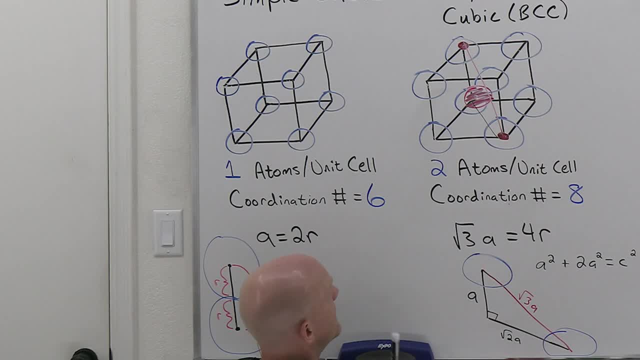 an atom that looks horrible at this corner, and then you had the atom at the body-centered position right here, And so you get once again got a radii there, a diameter here which is 2 radii, and another radii there, for a total of 4 radii, which is going to equal. 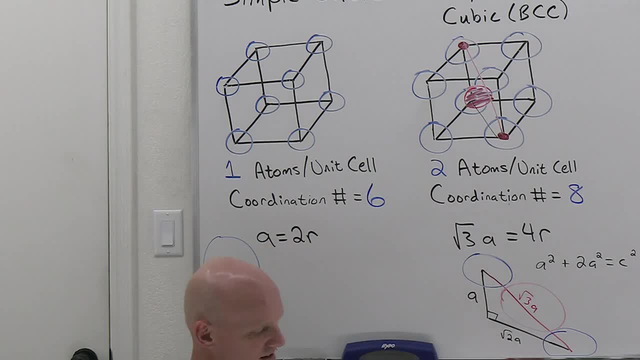 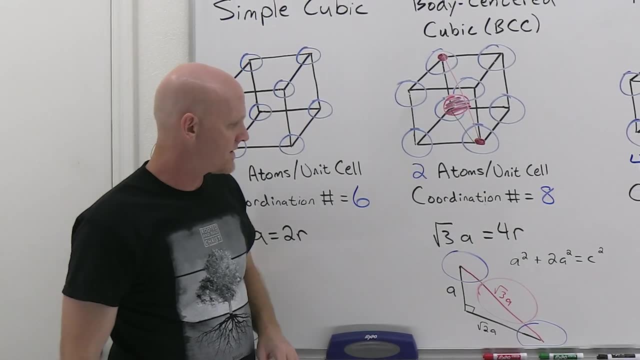 that square root of 3A along the body diagonal. So that's where that comes from. That's the one that students struggle with the most To see, So hopefully you can see it a little more easily here. But at the end of the day, 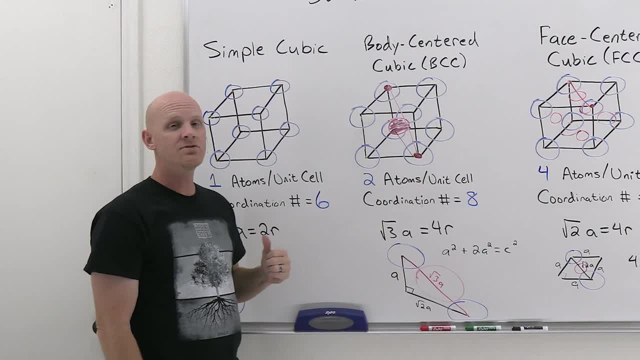 sometimes they're going to have you do some calculations here And they want you to. you know, if I give you the edge length, calculate the radius. or if I give you the radius, you know, of the atoms in the unit cell, calculate the edge length. And you just have to know the right. 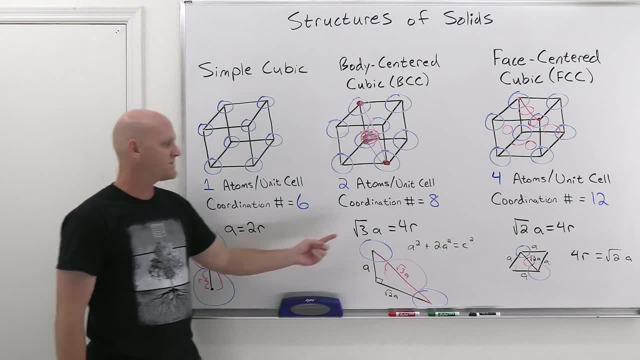 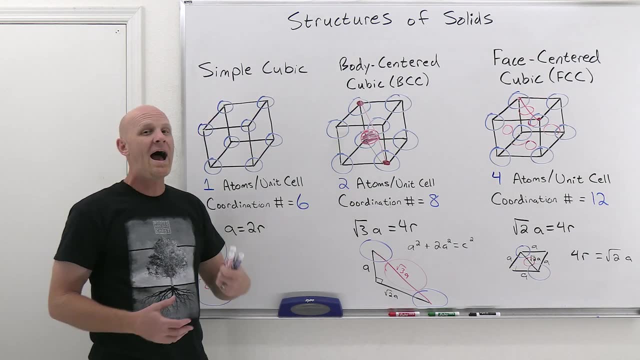 relationship. If it's simple cubic, obviously you've got the easiest relationship, but if it's body-centered cubic or face-centered cubic, they'd give you one of these other relationships. Now we can also talk about what's called the packing efficiency And generally, as you go from 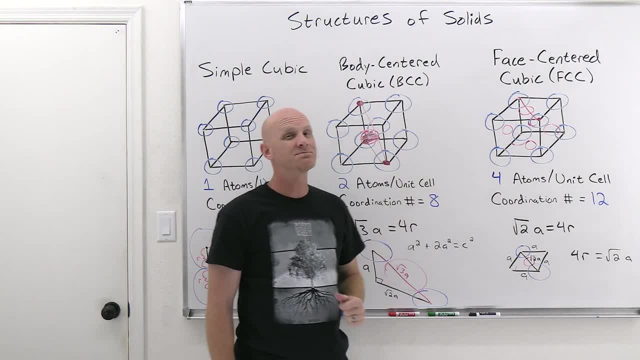 simple cubic to body-centered cubic. you have to be very specific here. If you're learning theèseum, you're going to have to be real, specific And just for the sake of my talking, I was thinking about this today- to body-centered cubic to face-centered cubic. this packing efficiency is going to increase. 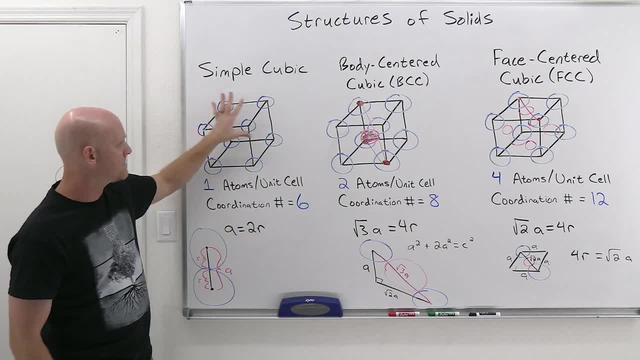 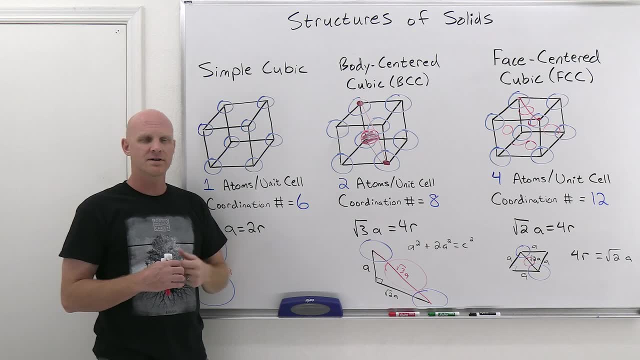 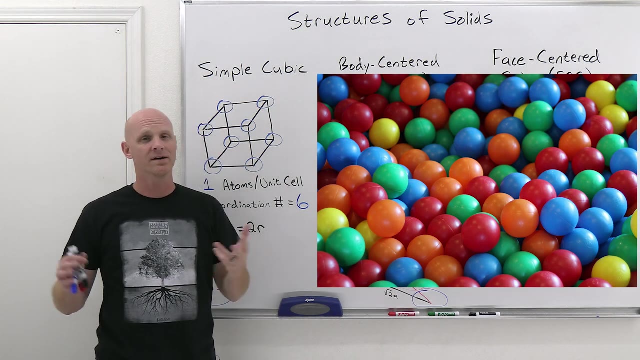 And ultimately what that packing efficiency is. it is the percentage of the volume of the cube that actually has an atom in it. So note, if you try to take some of these, maybe that big pool full of hollow plastic balls maybe you played with as a kid. they don't really have them anymore. 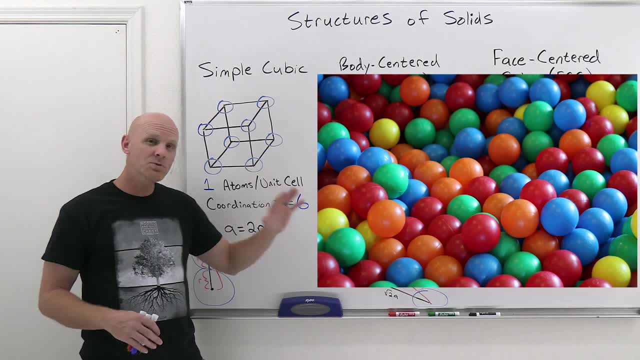 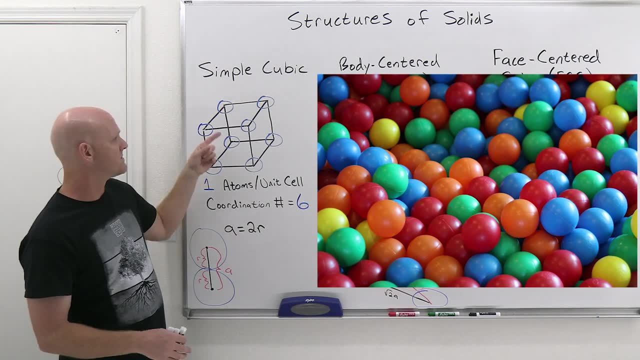 because they're germ fests and stuff like this. But maybe you played with those as a kid. you jump into this big pool full of these hollow plastic balls and think about that kind of like this And there's a lot of empty space in there. So because, being spheres, there's just going to 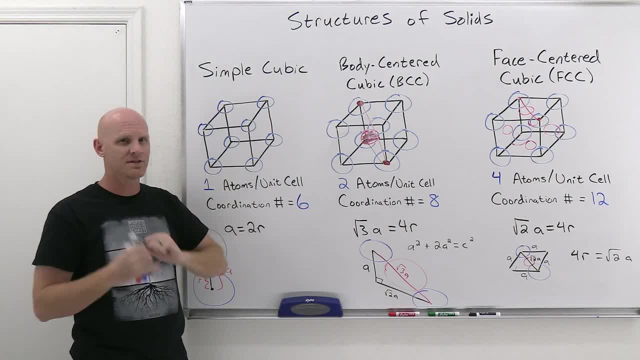 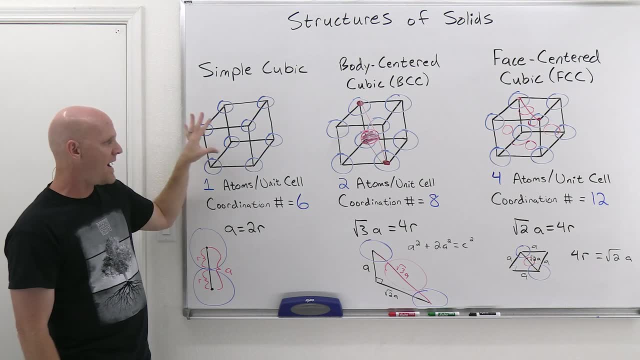 be some empty space. You can only put them so close, And once they even touch there's just a lot of gaps in there and stuff like that. And so same thing is true in these unit cells with our lovely spherically shaped atoms, And so the packing efficiency is just going to be a measure of what. 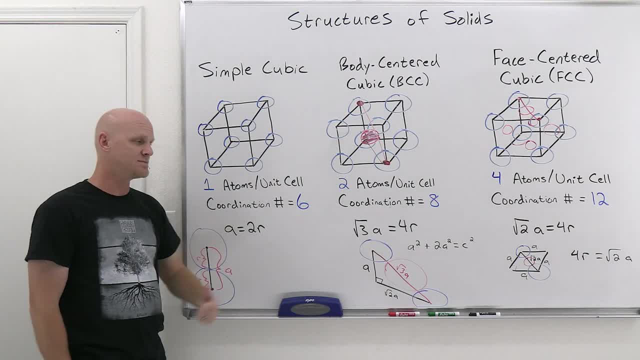 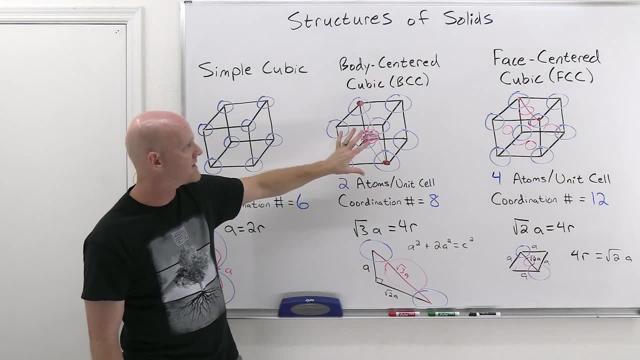 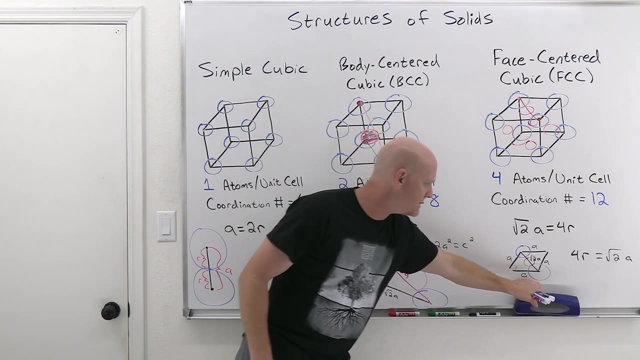 fraction of the unit cell is occupied by atoms instead of empty space. And it turns out it's going to be 52% Packing efficiency for the simple cubic, 68% for the body centered cubic and then 74% for the face centered cubic. And if you look at how that calculation actually works, it'll definitely be. 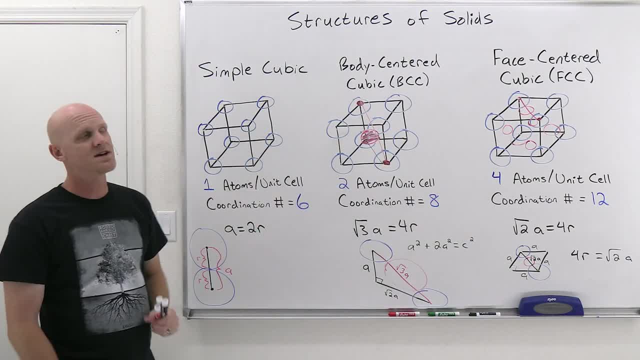 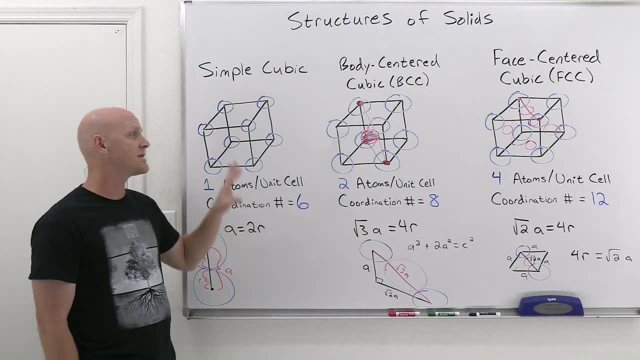 easiest to do for the simple cubic, But then when you could apply the same thing to the body centered cubic and face centered cubic? So what you want to do is take the volume occupied by atoms divided by the total volume of the unit cell times 100. And so in this case, with one atom per unit cell. 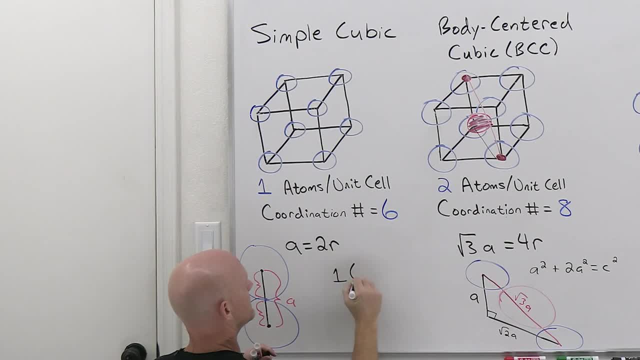 it's just the volume of one atom per unit cell. And so in this case, with one atom per unit cell, well, the volume of a sphere is four thirds pi r cubed, So it's just one sphere. So for the body. 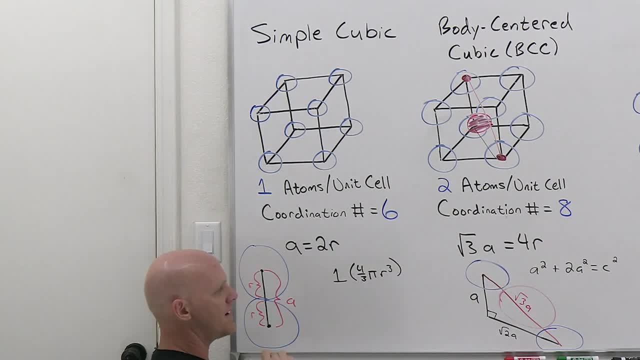 centered cubic, you'd have to multiply that by two. And for the face centered cubic, you'd have to multiply that by four. So, but in our case it's just that, and then divided by the volume of a cube, Well, the volume of a cube is just a cubed, And then you multiply by 100.. So well, in this, 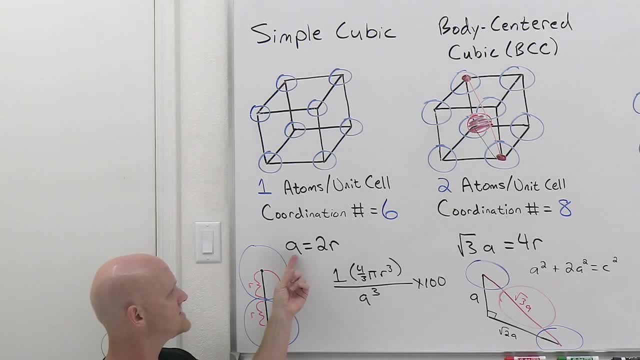 case, I've got two variables. I got r's and a's and they're not going to cancel. But what you could do is take and substitute for the a here two r, And so we'll take that a and erase it and substitute in two r in its place And you'll cube. 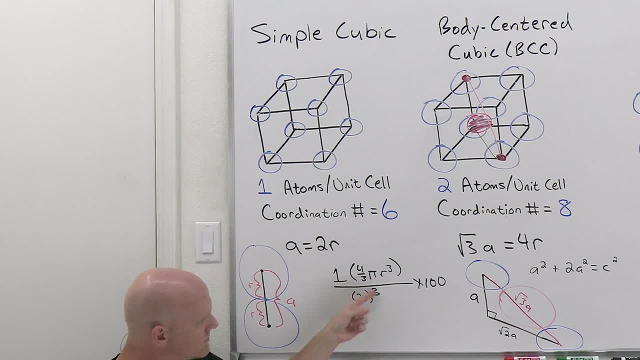 both the two and the r to get eight r cubed on the bottom, and then the r cubes will cancel And you could actually solve this out and it would equal 52%. You could do this. something similar here you'd have to. you know when, instead of with your a cubed on the bottom, you'd have to come out with 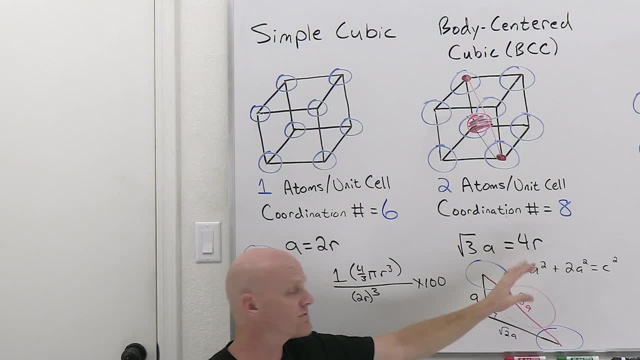 a slightly different expression for a. it equal four r over the square root of three. and then you'd have to cube it and stuff, But the calculation would be very similar And again you'd also have to factor in that instead of just one sphere you'd have two spheres in that body. 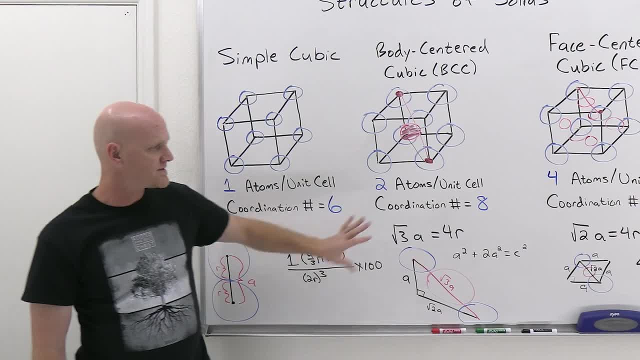 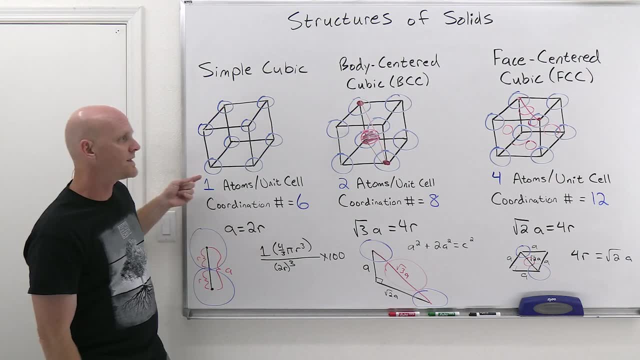 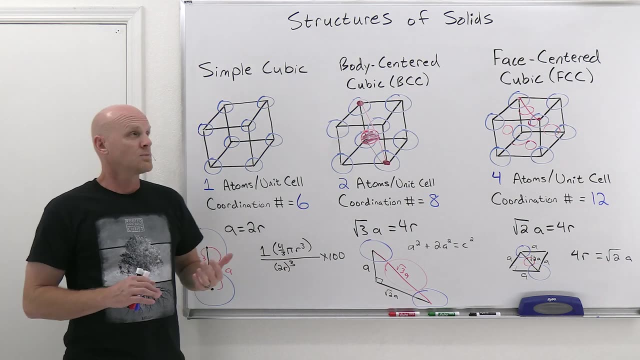 centered cubic and stuff like that. But that's where the 52%, 68% and 74% numbers and you may be asked to calculate those. So. but you probably should at least realize that the packing efficiency increases as you go from simple cubic to body centered cubic, to face centered cubic- Cool That's. 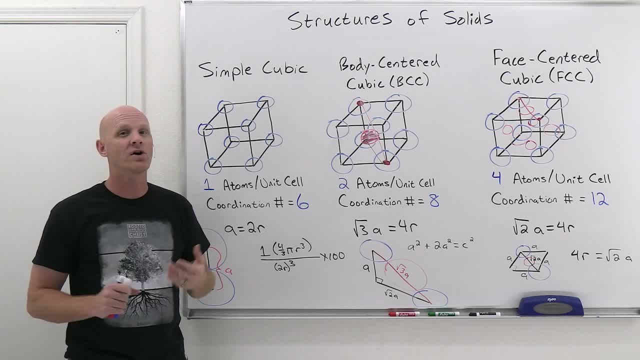 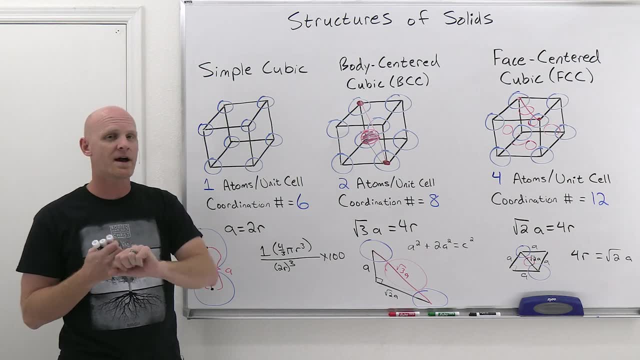 all I really want to say about these cubic unit cells. We now got to talk about our cubic- I should say- packing of spheres, both hexagonal close packed and cubic close packed. We'll see how these work. So now we're going to take a look at the close packing of spheres. in there Again, there's 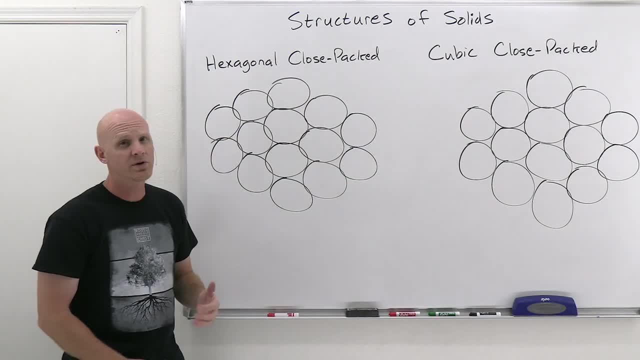 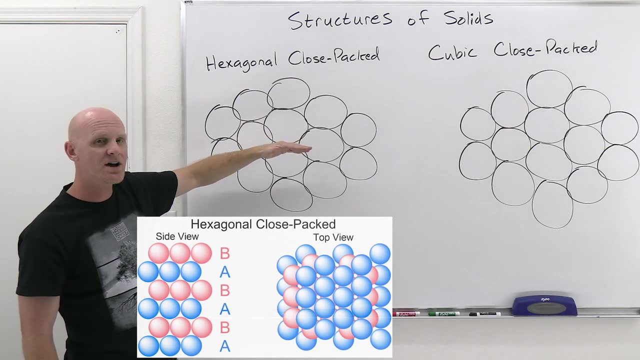 two types: hexagonal, close packed and cubic, close packed. And you'll notice that we're going to draw multiple layers onto this and a couple different perspectives. we'll look at the kind of a top down view, but then we'll kind of pull it off sideways And you could look at, you know how, the layers. 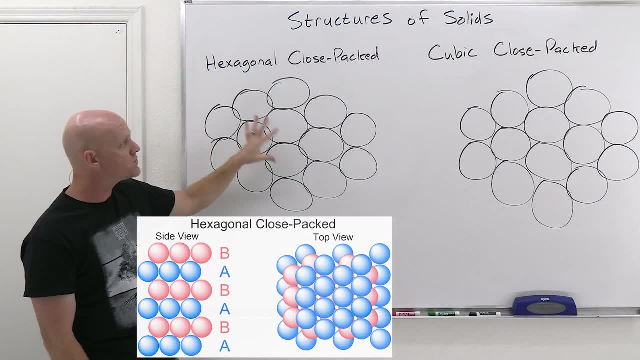 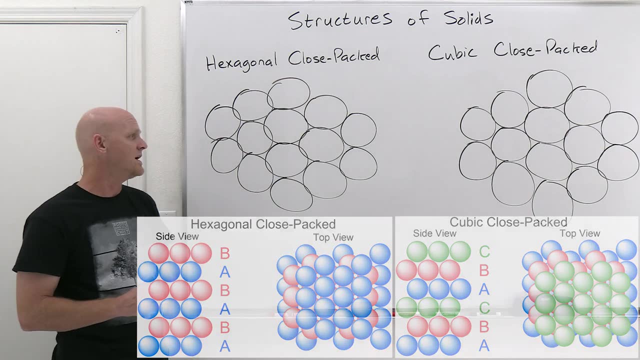 stack on top of each other And we'll find out really at the end of the day- is there's two repeating layers for hexagonal, close packed, where there's a set of three repeating layers for cubic, close packed. we'll see how this works Now. if you look at any single atom, you'll see. 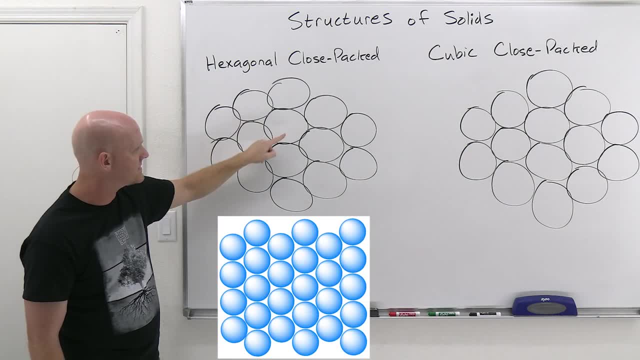 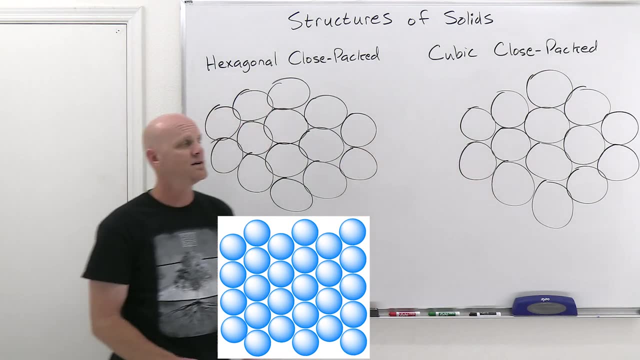 that it's surrounded in the same layer of atoms here by six nearest neighbors, kind of in the shape of a hexagon So, and that's true for both hexagonal close packed and cubic close packed. So, and the big thing is about, where does the next layer go on? And so we're going to put another layer on top. 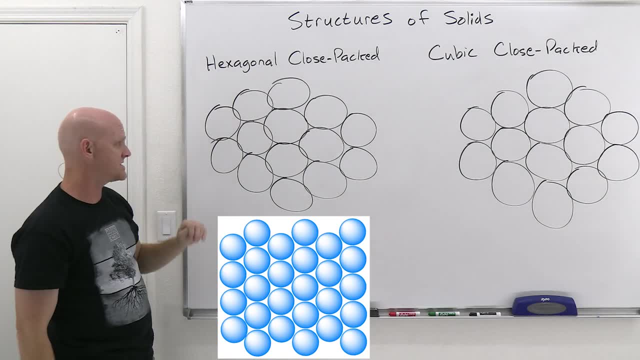 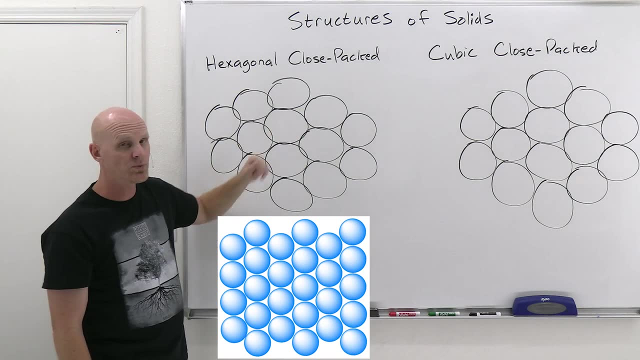 of this. So if we pull this outside, we can put another set of balls on top of this here, if you will. So another set of spheres. what you'll find out is that the next layer up wants to settle into these four gaps right here- or little holes, we might call them So- and there's two different ways. 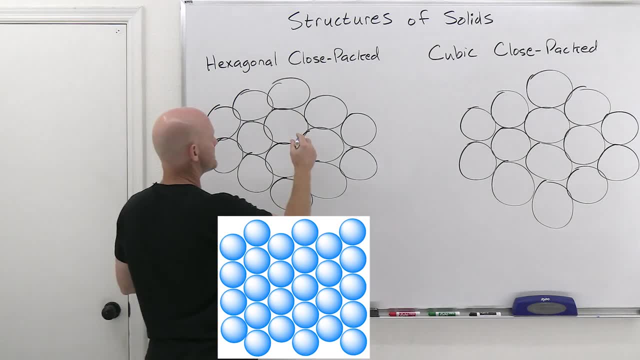 they could settle in there. And so in this next layer, let's say, we stick one of them right on this hole right here. So what you'll find out is that then the next one over here is going to settle on this hole right here, And then the next one down here is going to settle on this hole down. 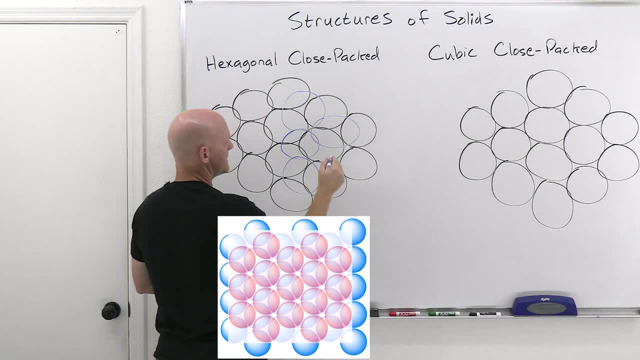 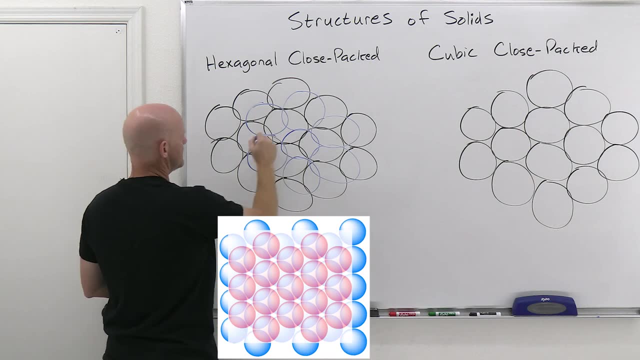 here, And then off to the right, you're going to have one centering on this hole and then one centering on this hole, And off to the left, here again one centering on this hole and then one's going to center on this hole, And so let's mark those holes. we got one. we'll just put an x there. 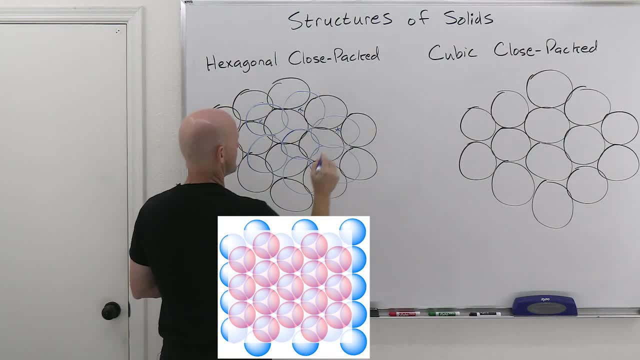 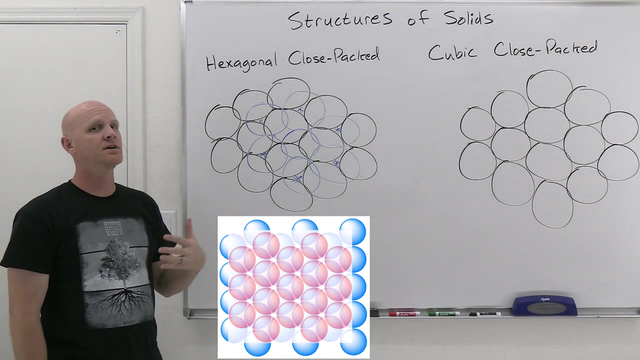 and there and there, there, there and there. So those are the six holes we centered the layers on, And so what you'll notice is that we haven't actually put spheres over all the layers. we have like a hole there that didn't get one on top of it, one there. 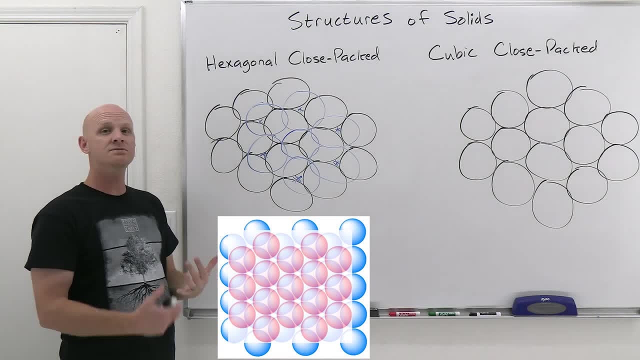 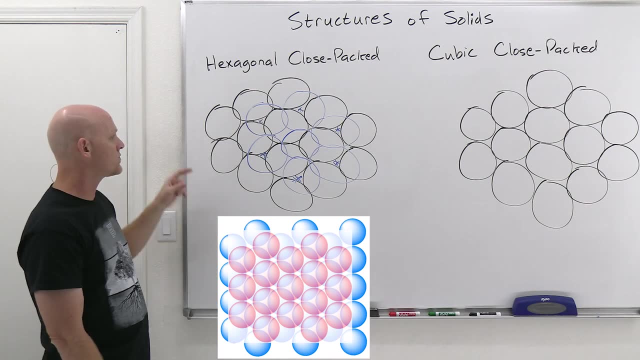 one there, one there, and so not all the holes actually have room to get a sphere, And so the question really becomes: okay, now what do we do with the third layer? Well, if we put the third layer right back where the original layer was. so notice, in the blue layer, there's a hole, right. 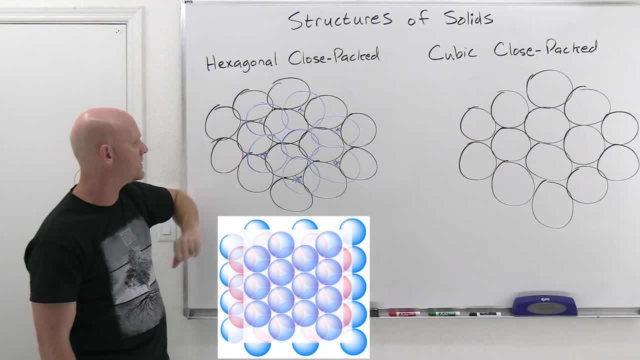 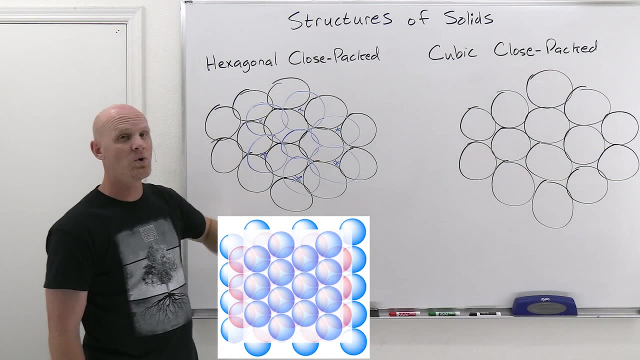 here we could just put a black sphere centered right on that hole. So there's also a hole right here and we could again put a black sphere right on top of that hole in the blue layer. And if we just go back to repeating the first layer, 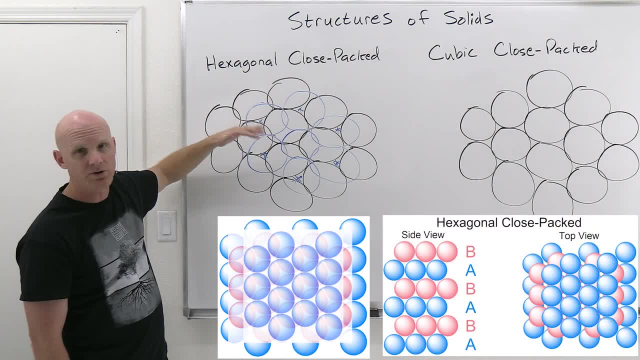 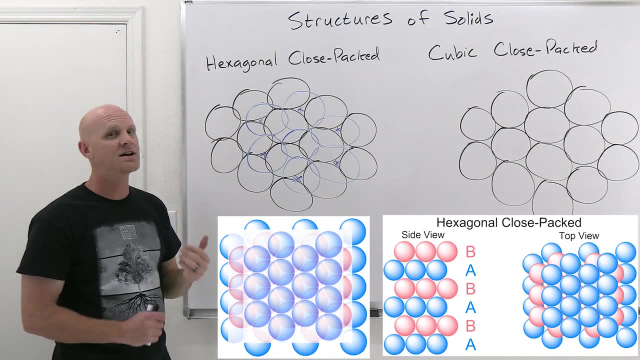 and then go back to repeating the second layer, so it's like black then blue, then black then blue, and just alternate those two layers all the way up. as you stack these spheres up, what you'd find out? that's actually what's indicative of hexagonal, close-packed. So what? 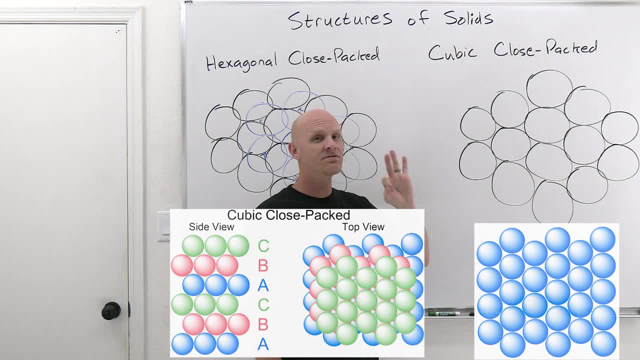 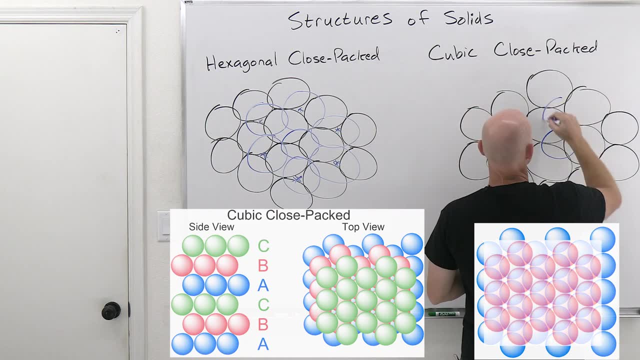 you're going to find, though, is that in a cubic, close-packed, you'll have this alternating set of three different layers, So let's draw that second layer in yet again real quick. So we've used this one, we've used this one, this hole, this hole, this hole and this hole, Oh. 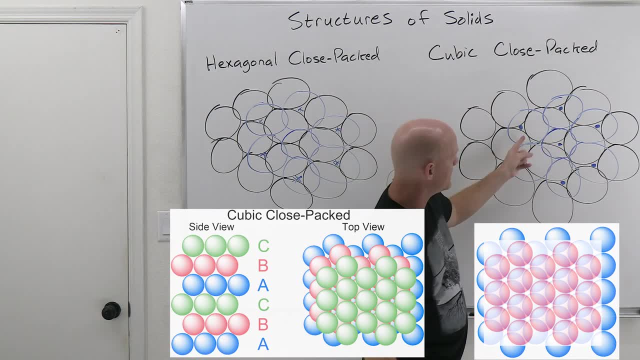 and then obviously the one in the middle- Cool. So now we've got the one in the middle and surrounded again by a hexagon. But there were certain holes that we didn't use. and we didn't use this hole right here And notice that's not only a whole in the black layer, it's also a hole in the 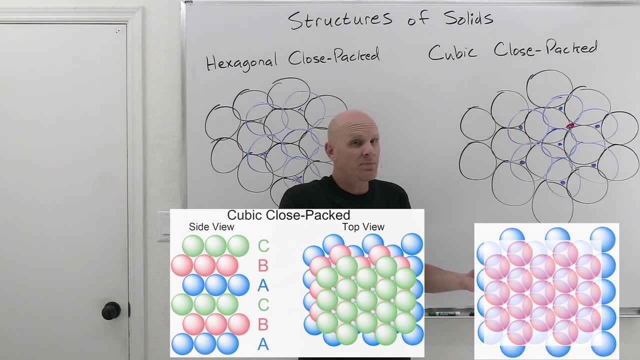 blue layer. it's one big hole right here, and so we have another place where we could put them, so we could replete the black layer over again, because that's going to be a hole for the blue layer as well. but we see that there are other positions here now that we can put atoms and if we create. 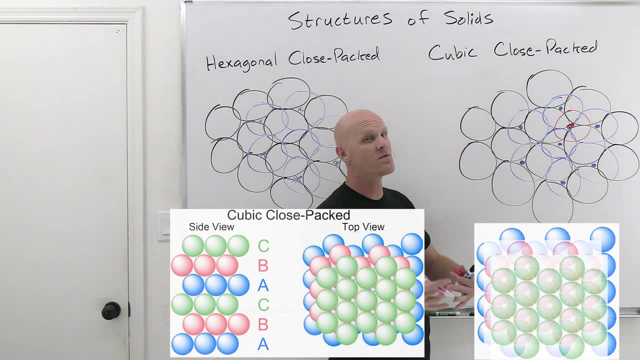 this new hole that's never been used and put an atom centered over that hole. that's going to be that third layer, and so once again we have an atom centered right there. so we also have another hole right in this region where another atom would get centered as well. we have another hole right in 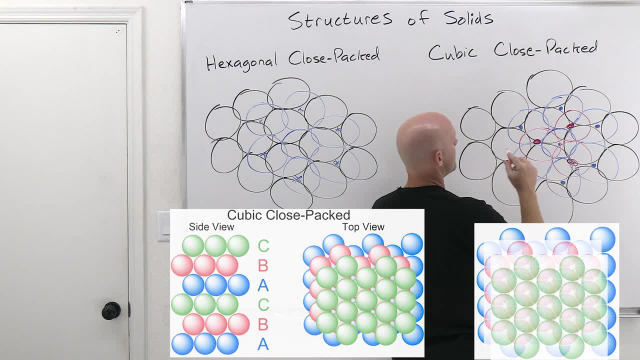 this region where another atom would get centered as well, and we could work our way all the way around in doing this kind of a thing as well and get six worked around him. and my drawing here is going to suck and I apologize, so the one I put up on the screen from the study guide is going to 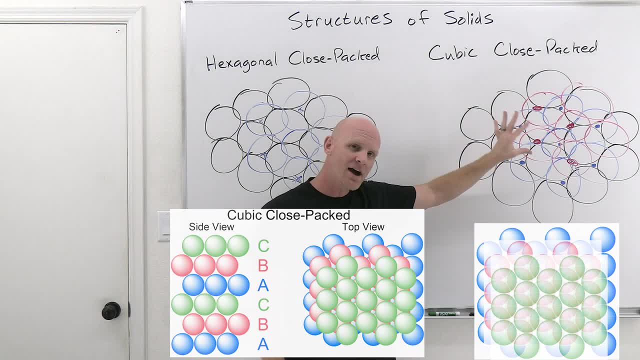 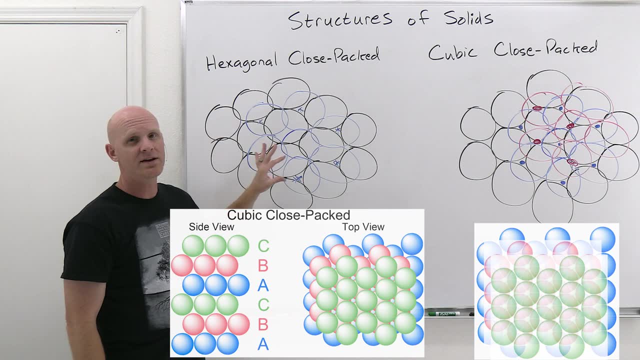 look way better than this. so but the big thing is, even if you can't quite see it, hopefully if you can, that helped a little. but even if you can't, the big thing to take away is that in the hexagonal close back you have two repleting layers. we might say like a, b, a, b. 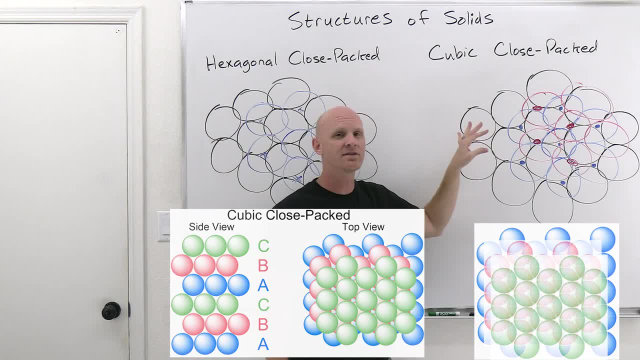 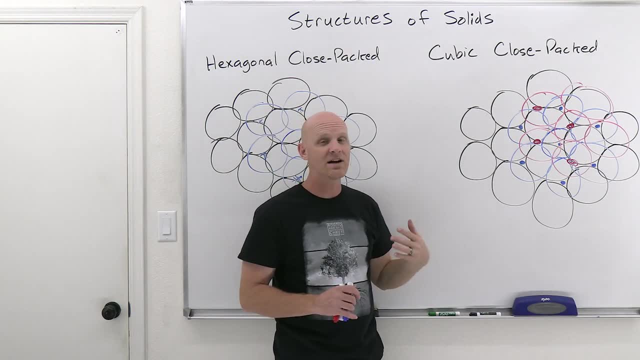 whereas in the cubic close pack there's alternating set of three layers, so A B C, A B C, so on and so forth. So that's your big difference here. but both of these have fairly good packing efficiencies. 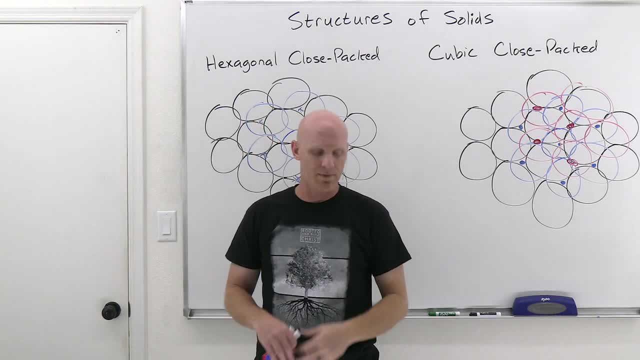 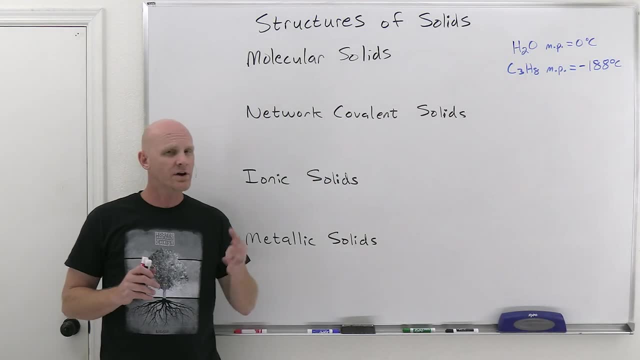 They're both really common in metals and things of this sort for pure metals to adopt these kind of structures and things of that sort. Alright, let's take a look at bonding and solids. So we'll take a look at our four different types of solids. 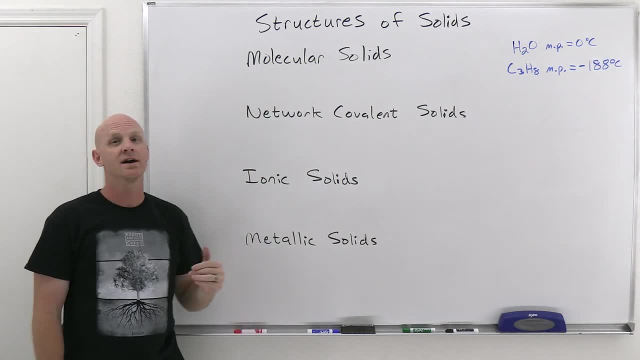 So we've got molecular solids, network covalent solids, ionic solids, metallic solids- and we've talked a little bit about each of these in earlier chapters and generally the way it works, the stronger the bonds or interactions holding these solids together. 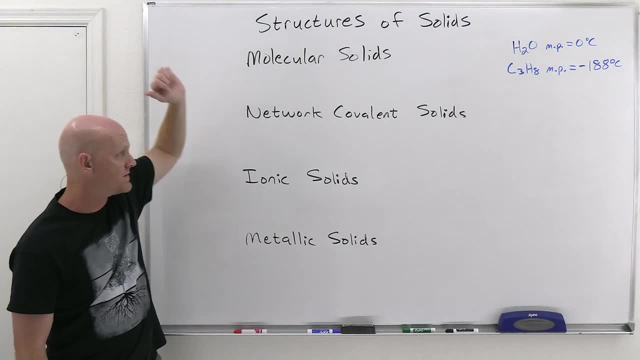 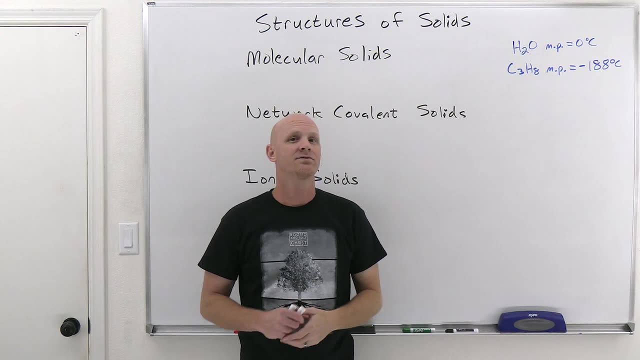 so the higher the melting point. So we'll start with molecular solids and we could talk about something like ice, and ice has got a melting point of zero degrees Celsius and it turns out that's rather high from molecular compounds. So molecular compounds in general tend to have fairly low melting points. 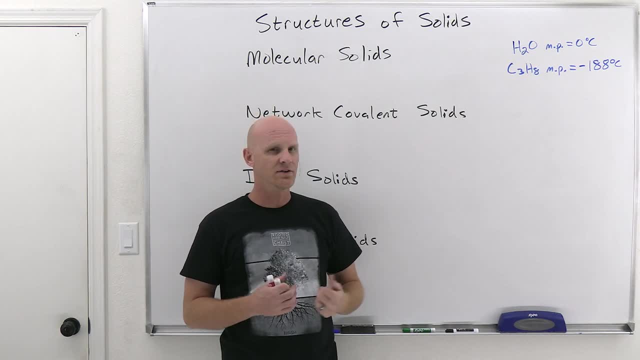 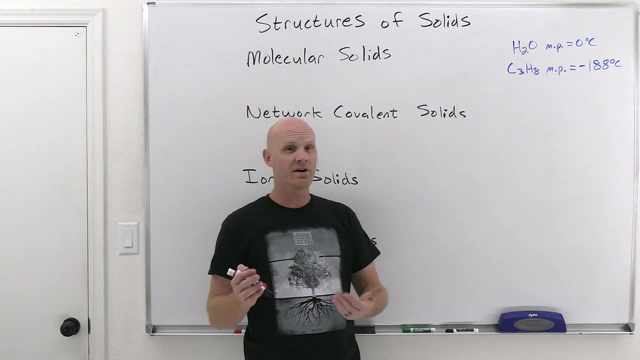 and the reason is: what's holding them together these solids is not bonds, It's actually just intermolecular forces which, you might recall, are much, much weaker than actual ionic or covalent bonds, And so, as a result, they melt at much lower temperatures than a lot of the rest of these compounds. 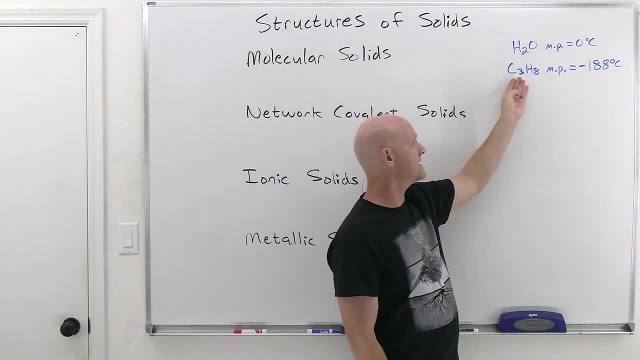 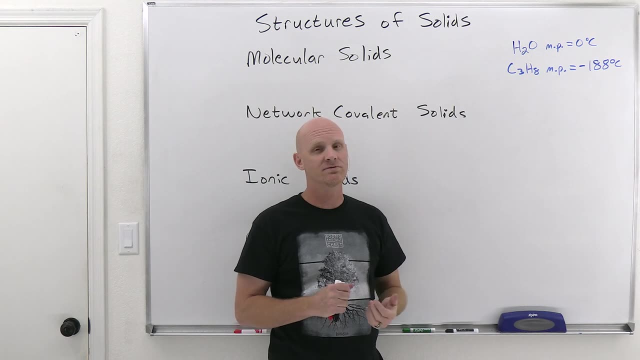 especially the network covalent ionic, as we'll see. So if you take a look at propane here- C3H8, its melting point is negative 188 degrees Celsius. So in fact, at room temperature we're not only higher than its melting point, 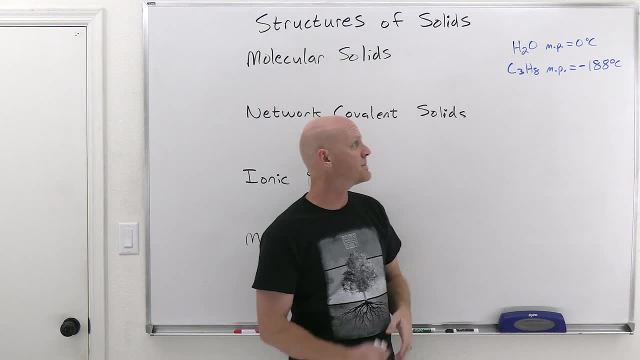 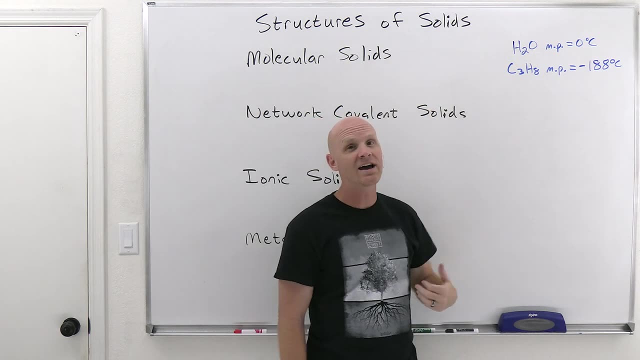 we're higher than its boiling point and it exists as a gas at room temperature and things of this sort. So just a couple common examples of molecular compounds. And again we learned with hydrogen bonding water's got a fairly high melting point and boiling point. 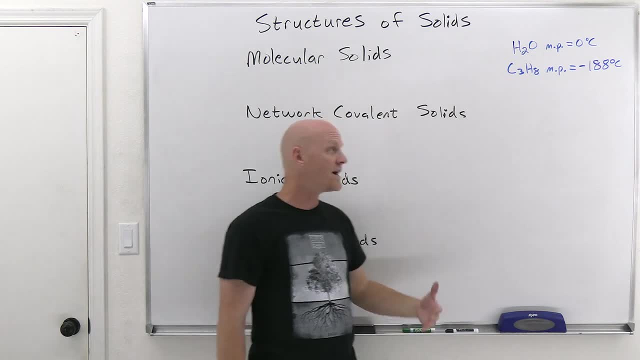 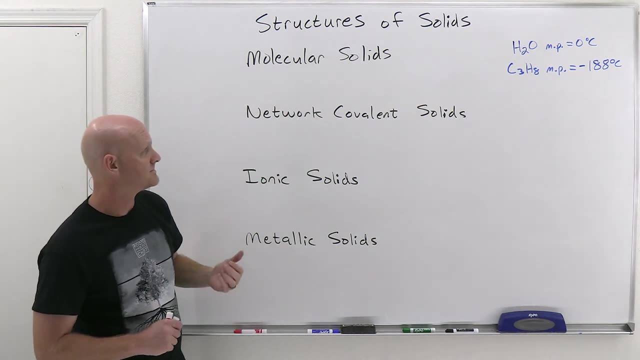 again compared to other molecular compounds. But now we're actually going to see that, comparing molecular compounds to some of these other types, we're going to see that they have relatively low melting points. So next we'll take a look at network covalent solids. 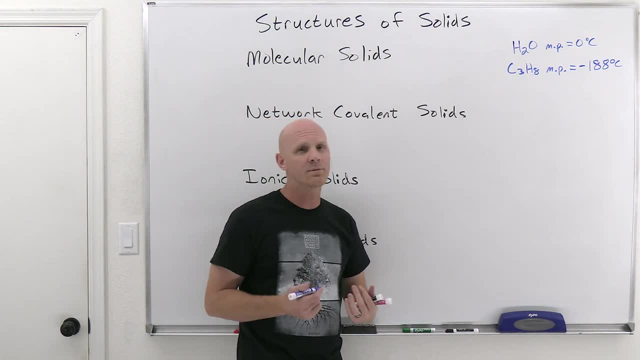 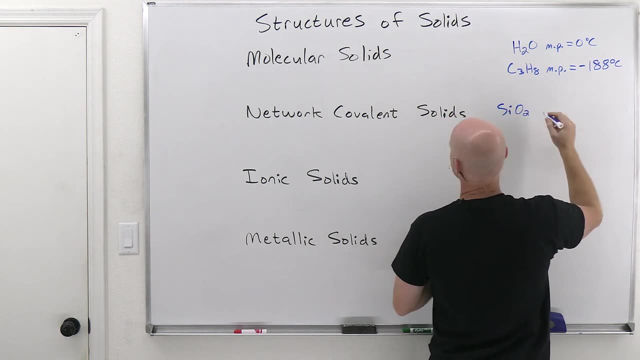 You might recall that diamond, graphite, both forms of solid carbon, and then silicon dioxide, quartz, both examples of these network covalent solids, And you're going to find out that they have much higher melting points. So right off your study guide, I think it's yeah, 1700 degrees Celsius. 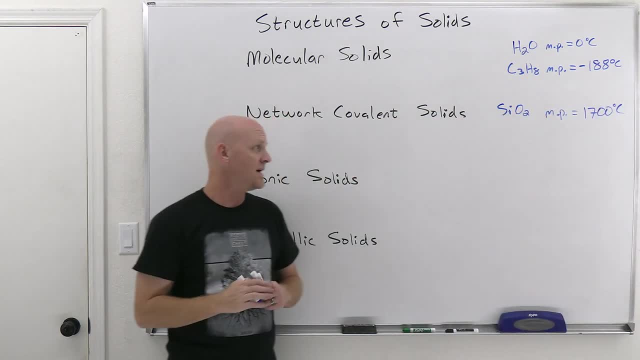 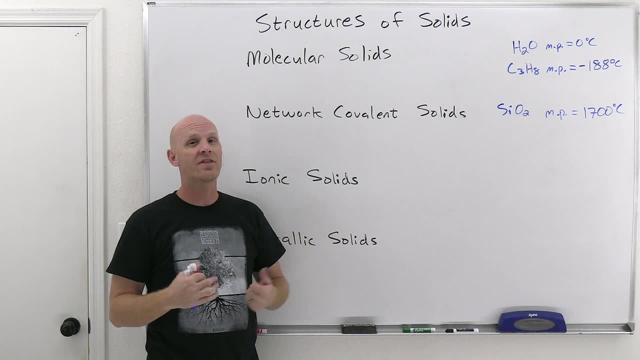 And diamond even higher than that for a melting point, And so the idea is that these are not held together. these solids are not held together by intermolecular forces. now, It's actually a crystal lattice held together by covalent bonds, And if you want to melt it, you've got to break some of those covalent bonds. 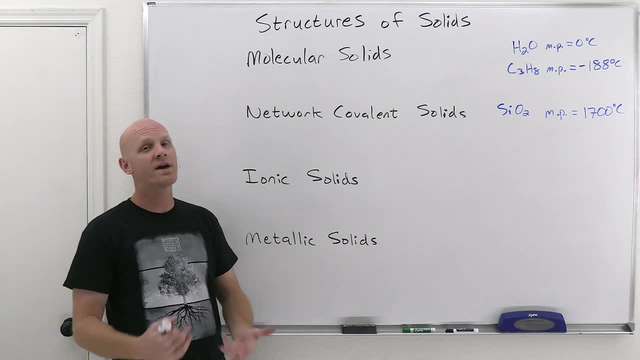 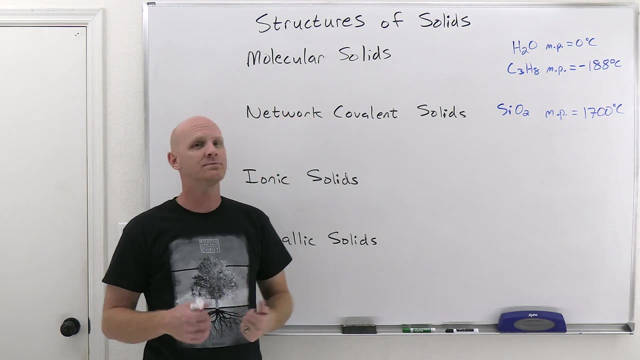 And since they're way stronger than intermolecular forces, it's going to take way more energy and happen at a much higher temperature, And so these network covalent solids typically have some of the highest melting points you're going to encounter. Like I said, diamond here, pure carbon, even higher than silicon dioxide. 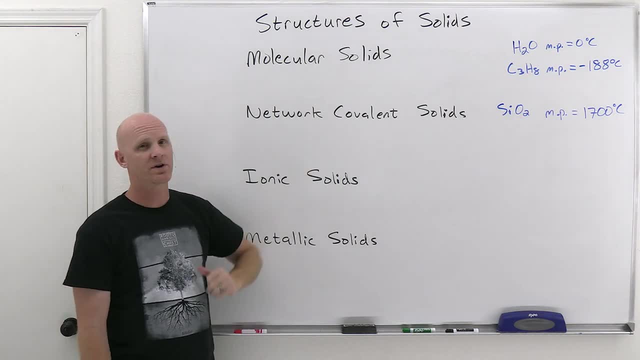 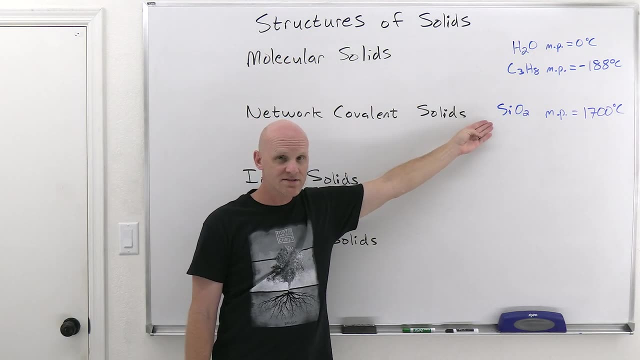 Cool, Then we'll move on to ionic solids. Notice, there's not a whole lot of these network covalent solids, So being made of nonmetals, usually that means you're going to be molecular, So carbon, diamond, graphite or quartz, in this case silicon dioxide. 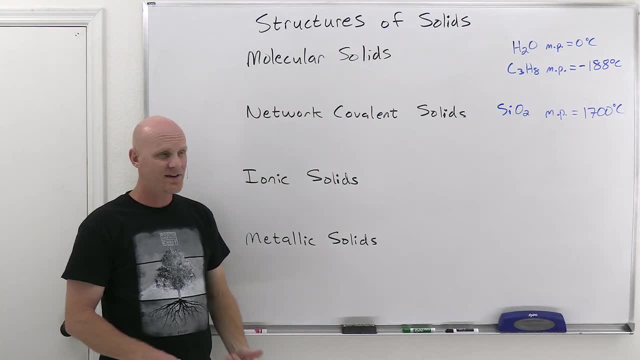 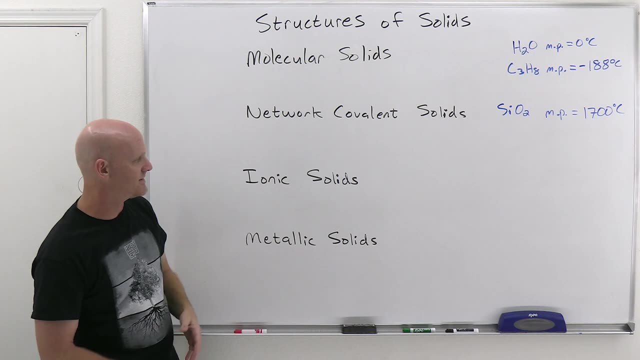 pretty much the three most notable examples you're ever going to encounter. Anything else you encounter that's made of only nonmetals is probably 99.9% likely to be a molecular solid instead. Okay, ionic solids. So ionic solids like metal and nonmetal, or it could involve polyatomic ions. 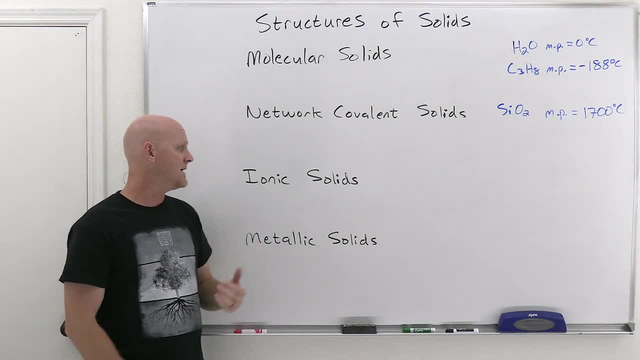 But the only ones we're going to specifically look at are going to be a metal with a nonmetal, And we looked at ionic solids. We looked at lattice energy way back in, like chapter 8 maybe, And with ionic solids it turns out the higher the lattice energy. 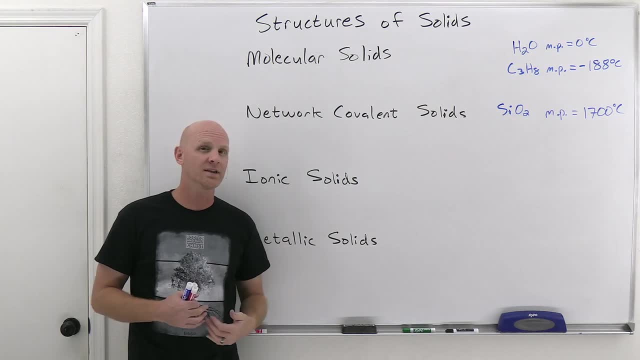 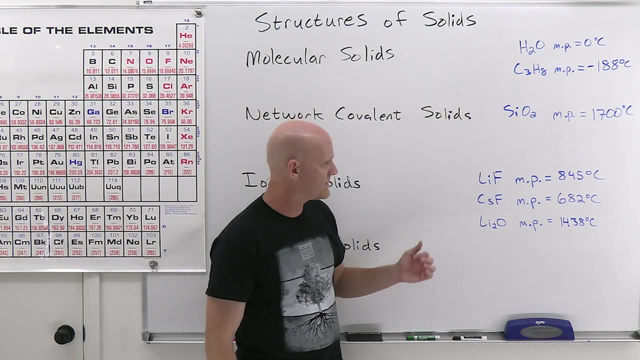 the stronger the ionic bonds holding it together, And now we'll see that we can also relate that to a higher melting point. Let me get a couple of them up on the board here. All right, so now we've got three ionic compounds up here. 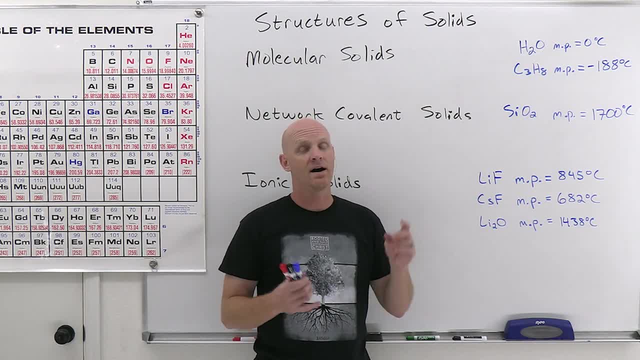 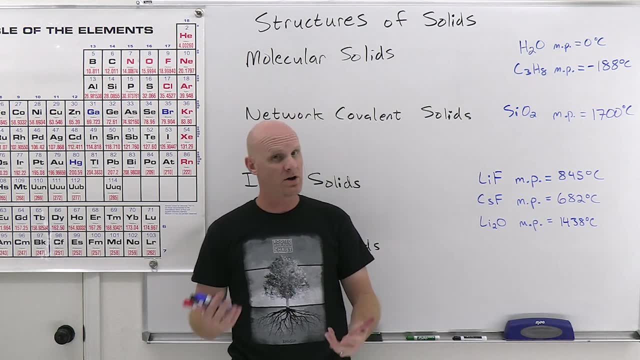 And you might recall that for lattice energy we said that larger charges and smaller ions make stronger ionic bonds and have higher lattice energies, And now we're going to also relate that to higher melting points here. So we take a look at LiF, CsF and Li2O. 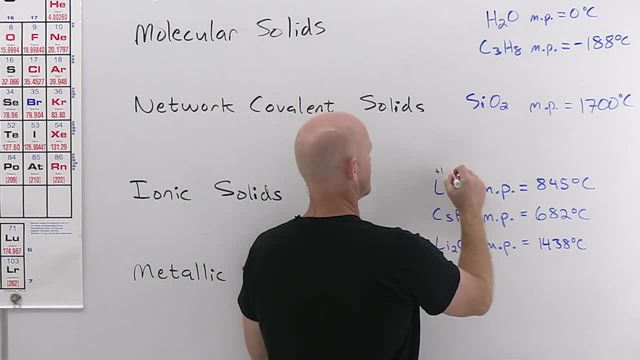 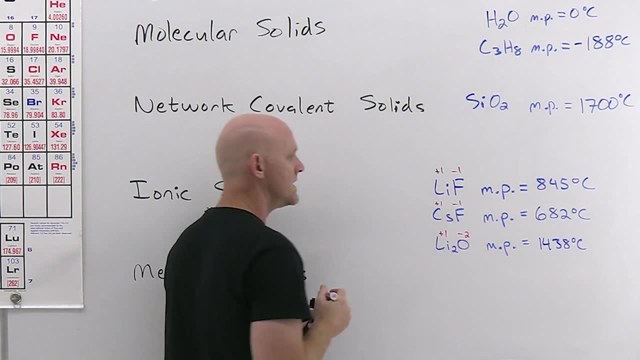 So we'll see that LiF and CsF both have plus 1 and minus 1 cations and anions, whereas Li2O has a plus 1 cation but a minus 2 anion And with that larger charge we expect it to have the highest lattice energy of the three. and therefore the highest melting point, which is exactly true. Notice it's considerably higher than either CsF or LiF. Now, in comparing LiF to CsF with lattice energy back in the day we talked about size, And smaller ions can form shorter ionic bonds. 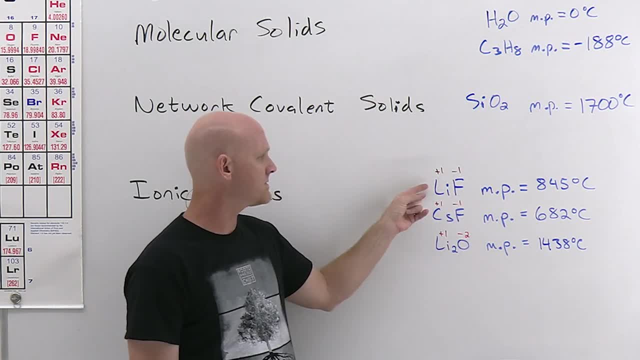 which are stronger ionic bonds, And so they both have fluorine in common. but it's the difference between lithium and cesium. And so if we take a look at the periodic table here and we take a look at lithium versus cesium, 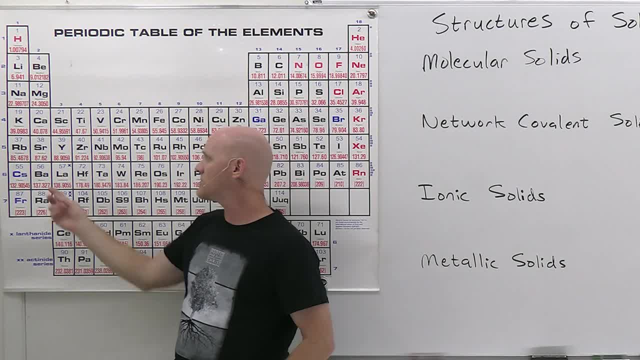 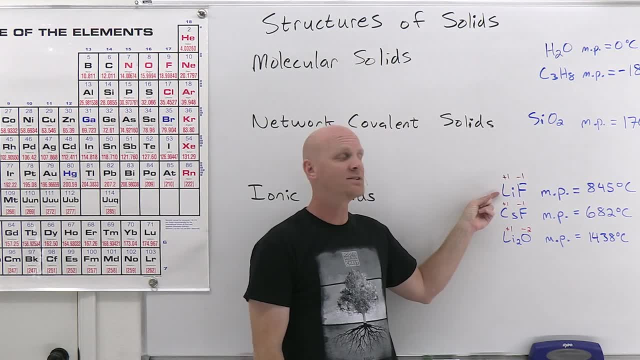 we see that lithium is significantly smaller than cesium And, as a result, lithium should make shorter ionic bonds, And shorter ionic bonds are stronger, which means a higher lattice energy and in this case, corresponds also to a higher melting point as well. 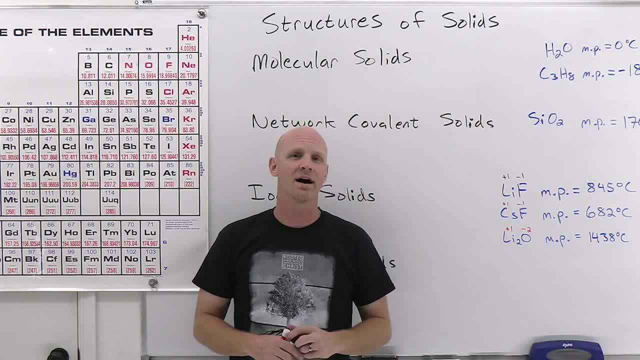 And so the same characteristics that led us to determine higher lattice energies are also going to lead you towards determining higher melting points for ionic compounds in this lesson as well. Now we'll finish this off by looking at metallic solids, And so metallic solids. there are some patterns here. 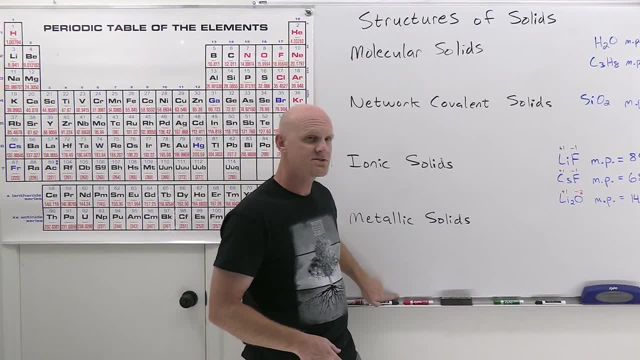 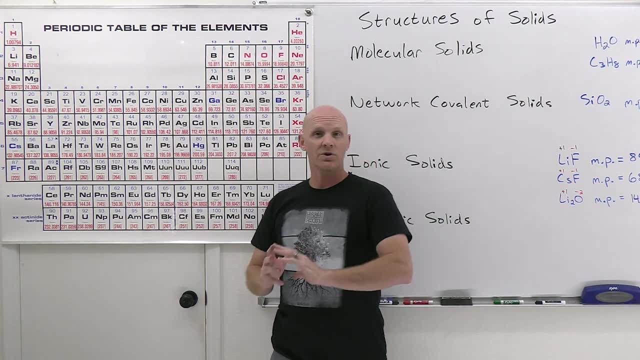 but this one's going to be a little bit challenging. So there's some funky stuff that goes on with some of like the transition metals and things of this sort. But if we take a look at just the main group metals for a second, if you recall, the metals are on the left-hand side of a staircase. 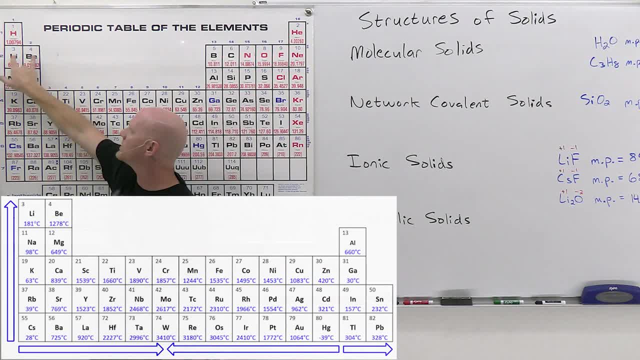 and stuff like this. So if we take a look at first just the alkali metals and the alkaline earth metals, we'll find out that the smaller ones are going to have shorter metallic bonds in this case, And have higher melting points as well. 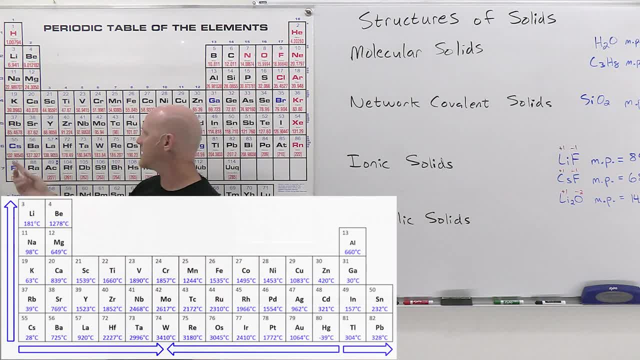 So as you go up a group you get higher melting points. So like cesium, it would melt in your hands, whereas like sodium, I think, is somewhere in the ballpark of like 200 degrees Celsius or something like somewhere in that ballpark. 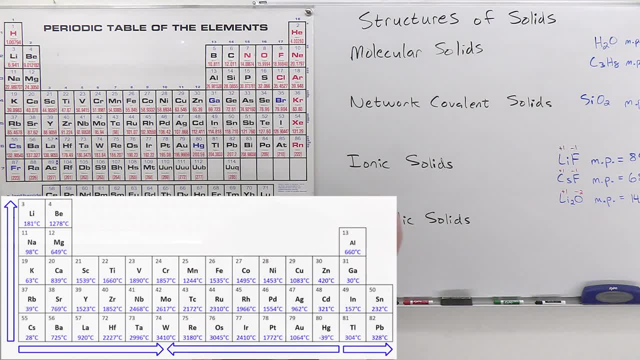 And on the study guide I put an entire list. In fact I guess we can look at sodium here. Sorry, sodium is 98 degrees Celsius. I am wrong there. But I put them on the study guide here a list kind of arranged by periodic table. 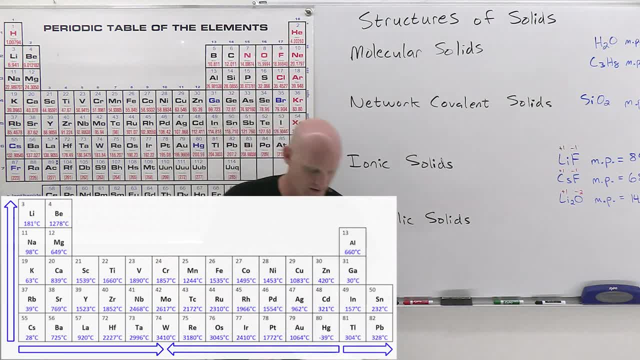 of some of the melting points of some of the metals. I'll put that up on the board on your screen there in a second Here as well. But you can definitely see that they go up. Melting points go up as you go up a group. 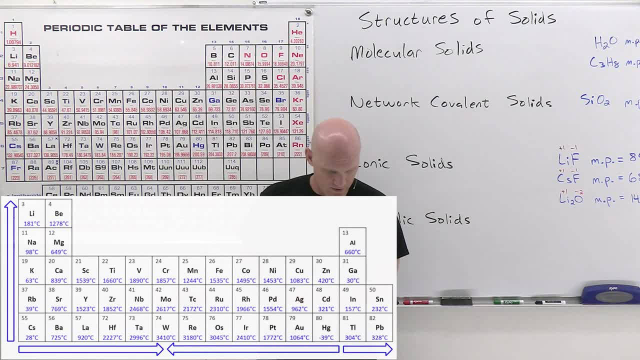 for the alkaline metals or alkaline earth metals. You'll also find out that as you go from alkaline metals to alkaline earth metals, you're going to have a higher melting point going that way as well, And the way it kind of works is: 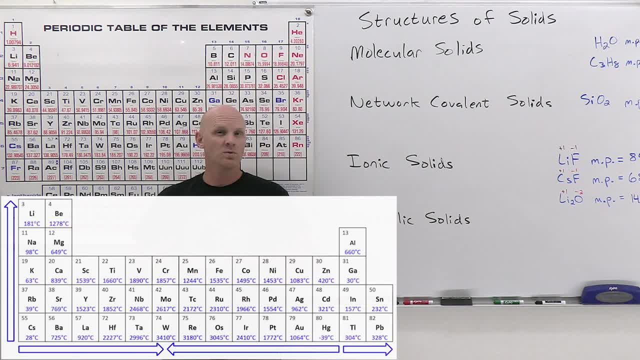 the more electrons that are available for bonding within the metallic structure generally, the higher the melting point, So that's part of it, And that's going to get a little bit tricky. when we start talking about the transition metals, though, because you might just think 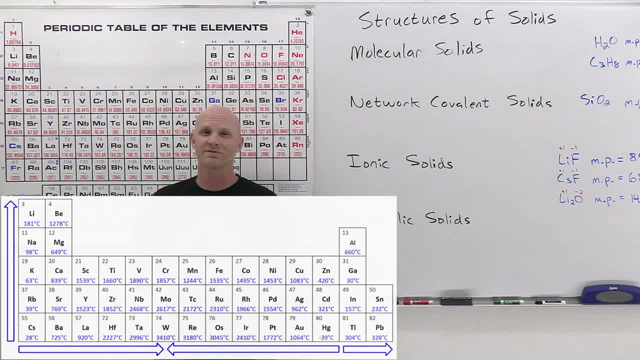 well then shoot. they should just increase as you go across, because you get more and more valence, electrons and stuff. But that's not entirely true, as we're going to see. Okay, So if we look at these transition metals over here for a second, 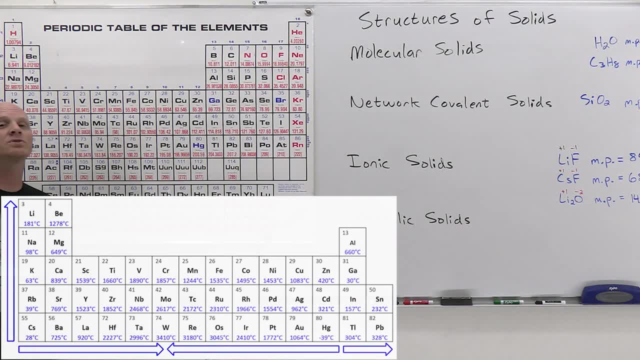 So we'll find out that the transition metals in the middle have the most unpaired electrons, And it's usually those unpaired electrons that are available for bonding, And so, within the transition metals, what you find out is that it's actually going to increase. 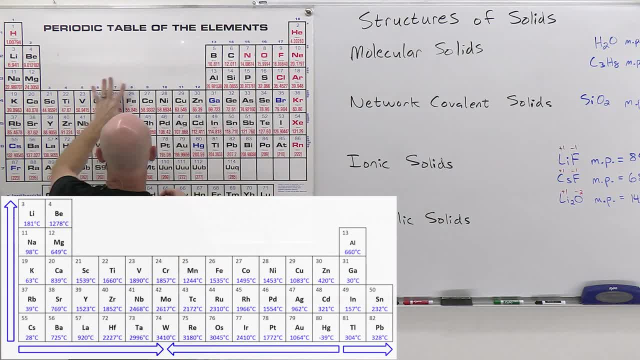 as you go left to right and right to left as you head somewhere towards the middle. So in here, And that's generally the trend And you don't have to get more specific than that, And it's not exact And there are exceptions to this and stuff like that. 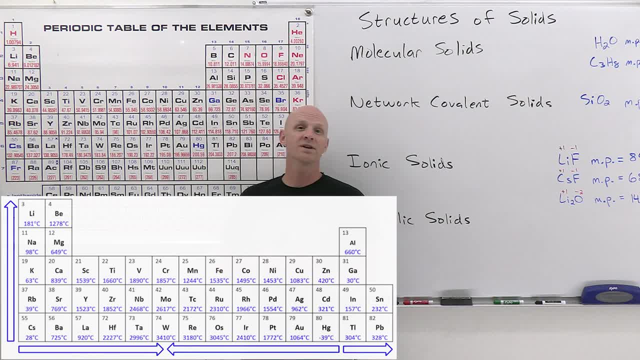 So, and you'll find that the vertical trend doesn't hold all that true either, So I wouldn't worry too much about the vertical trend. as far as the transition metals are concerned, You'll also notice a huge drop off when you go over here to some of these guys. 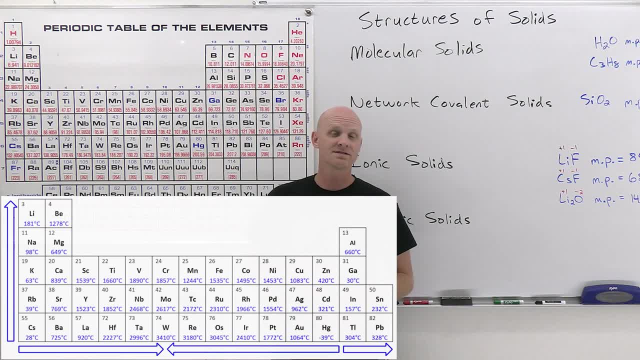 that fill up the d orbitals And those are no longer considered valence and stuff like that, And they're also not available then for metallic bonding, And so you get much weaker bonding right here with, like, say, zinc and cadmium Than you do with a lot of the other members in the group. 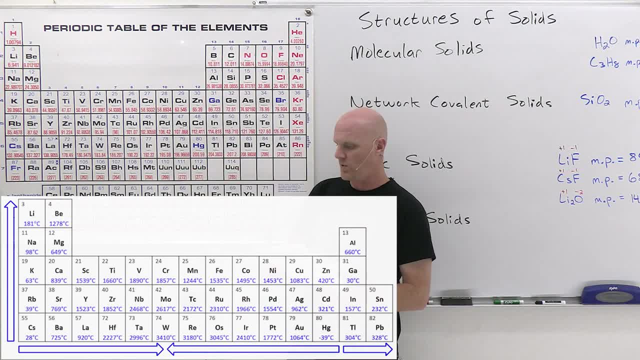 So, if you look at, like you know, zinc's got a melting point of 420 degrees Celsius, Whereas copper was over 1,000 degrees still And nickel's at over 1,400 degrees, But drops all the way down to like 420 degrees. 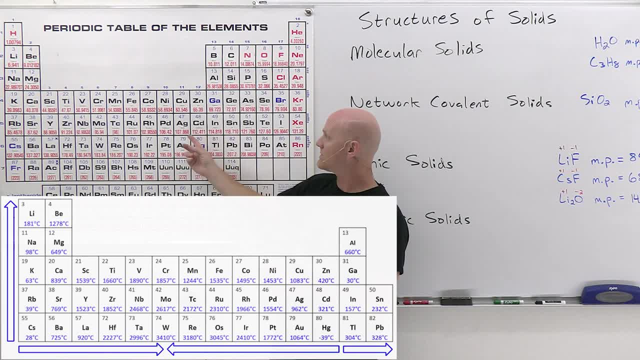 Cadmium same thing at 321 degrees, Whereas silver is just under 1,000 degrees And palladium was way up at 1,500 degrees. So huge differences there, and stuff like that as well. So and then, once you get to these few metals, 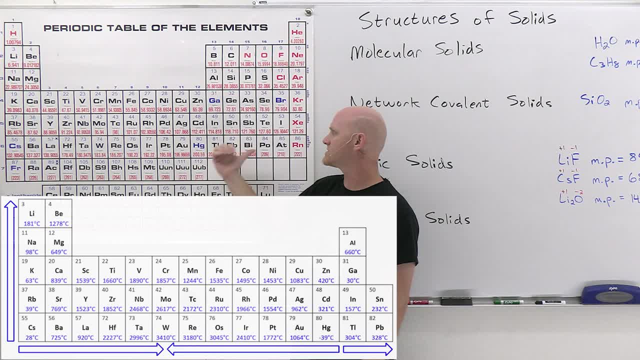 that are under the staircase here that are not. you know, once we get past the transition metals, they're going to increase, going to the right as well, as you get more valence electrons as well. So if we took out the transition metals, 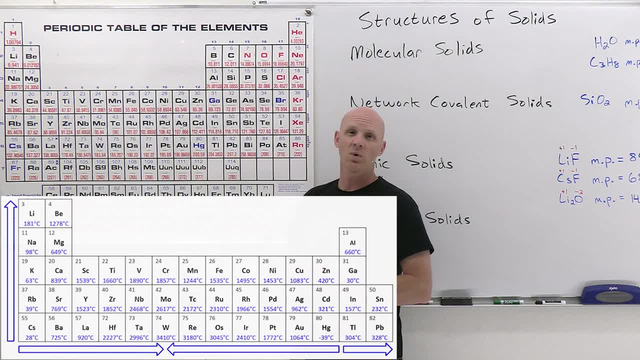 you'd be like: well, as you go from left to right you're going to get, you know, higher melting points with more valence electrons. But if you factor in those transition metals, you got to give them their own trend. 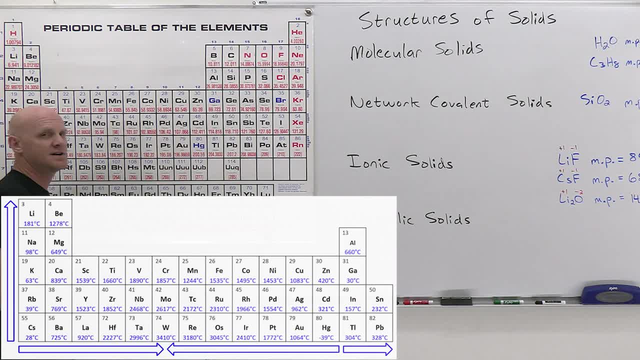 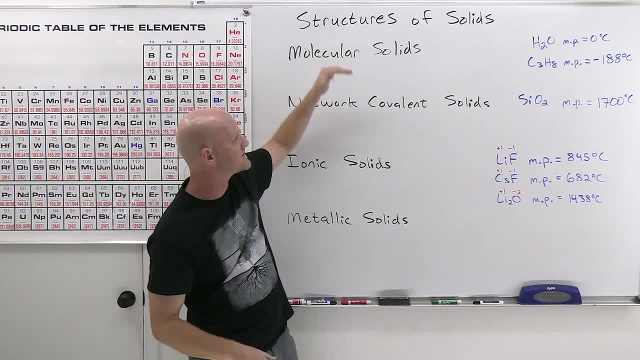 And again they're going to get higher melting points as you kind of go towards the center of those transition metals. Cool, And this is kind of the set of characteristics you're supposed to understand regarding these solids in this chapter and relating it to melting points. 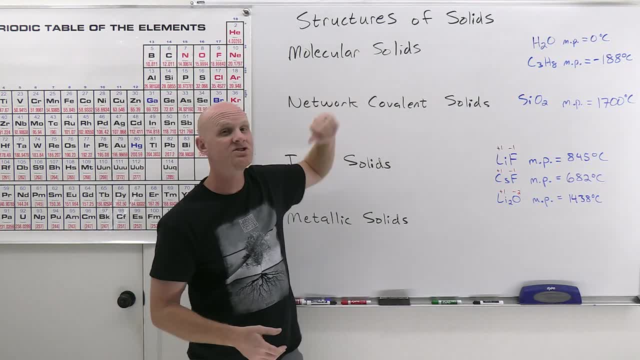 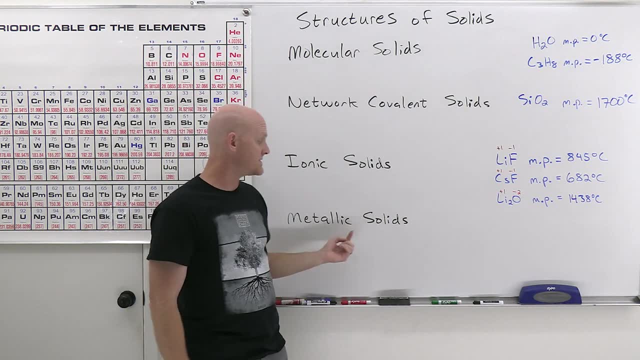 So once again you should realize that molecular solids generally are going to have some of the lowest melting points of any of these compounds. But don't forget that there are some solids, or some metallic solids I should say, like mercury, that actually you'd have to even cool it. 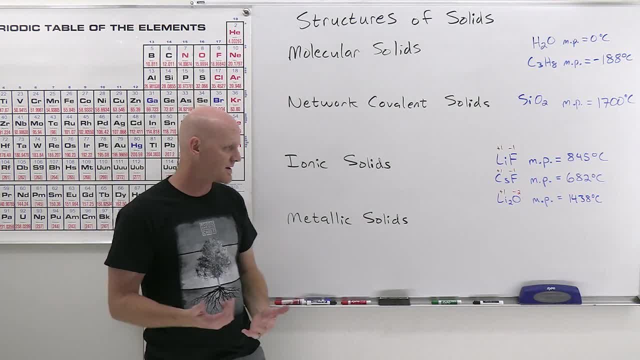 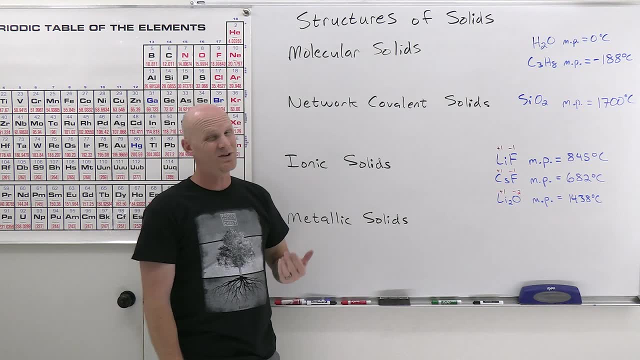 from room temperature. significantly, It's a liquid at room temperature and stuff. So don't think that all molecular solids are going to have lower melting points than all metals, for example. So there are also such thing as ionic liquids, although they're super rare. 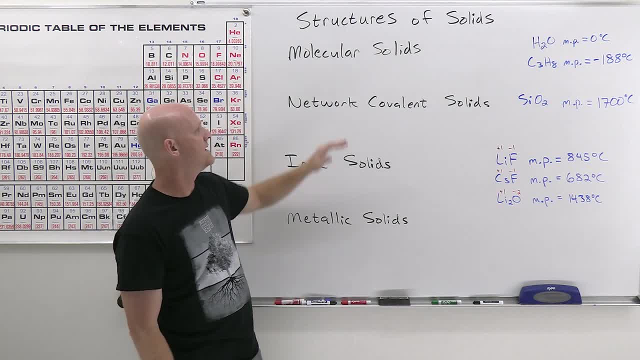 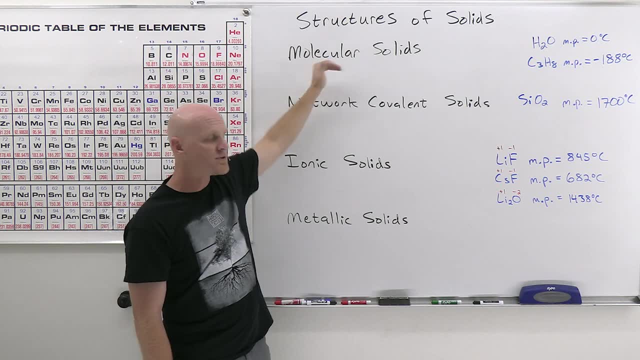 and I doubt you're going to see them. So you should generally consider network covalent solids to have the highest melting points, but ionics are a very close second, And then molecular solids are going to usually be in last place, And then metals. there's a pretty broad spectrum. 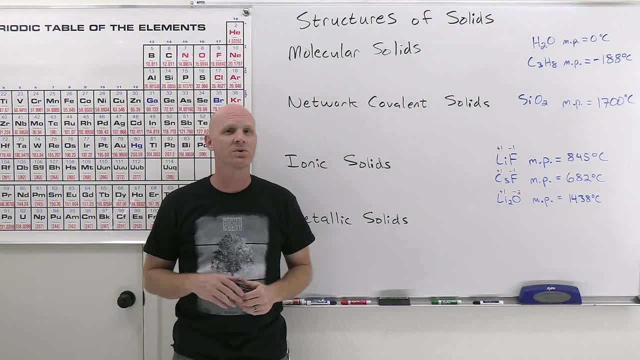 but notice, like iron and things of this sort, And we saw palladium was like 1500 degrees. Generally, a lot of them have fairly high melting points, But don't forget some of them, don't? So a lot of your alkali metals. 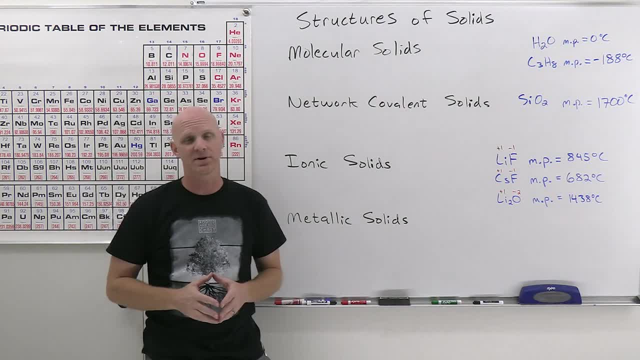 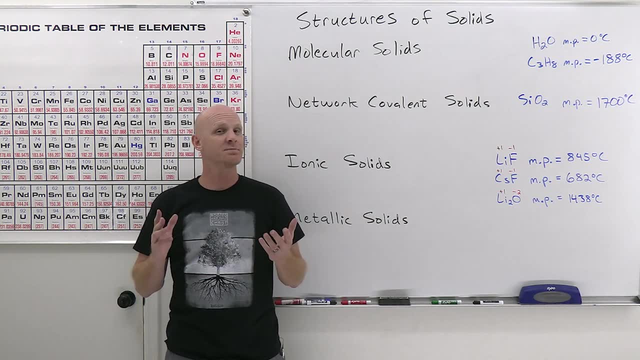 especially some of these larger ones, will melt in your hand and things of this sort. Now, if you found this lesson helpful, a like goes a long way to making sure YouTube shows this lesson to other students as well, And if there's something in particular. 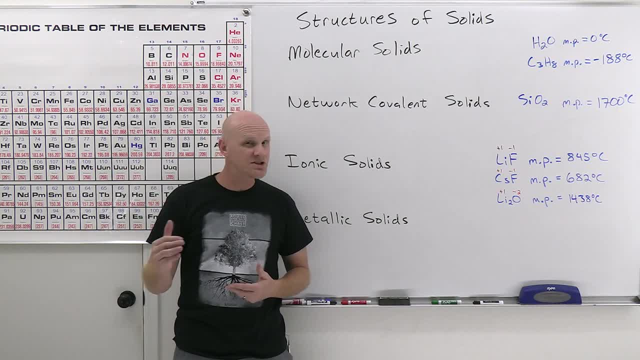 you liked about it, let me know in the comments below. If you think there's something I left out that you need to know. also, let me know in the comments below. I have been known to make supplementary videos here and there as well.